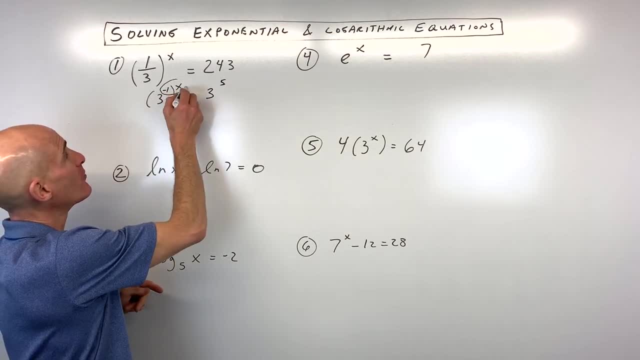 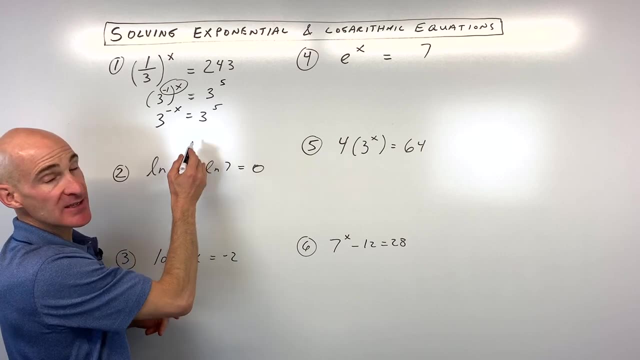 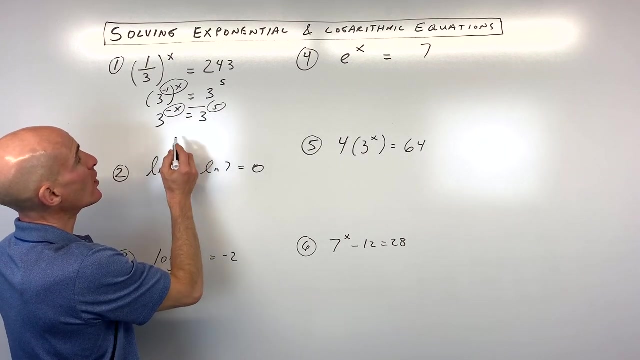 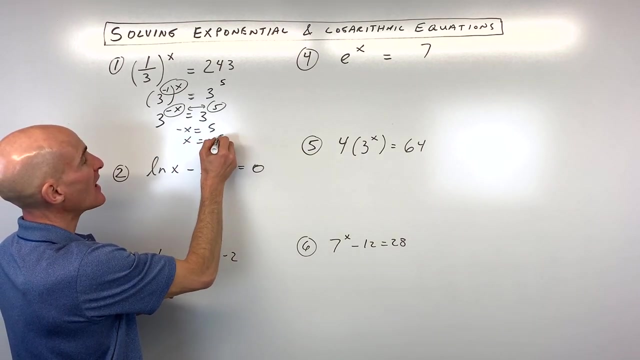 Okay, because that's the reciprocal. And remember, when you have a power to a power, what do you do to the exponents? you multiply them, And so now you can see we have the same base. this is what's called the one to one property of exponents. you can just set the powers or the exponents here equal to one another. So what I'm going to do is I'm going to say negative x equals five, multiply both sides by negative one, So you can see x equals negative five And that's your final result. Okay, let's go to number two. So this is a 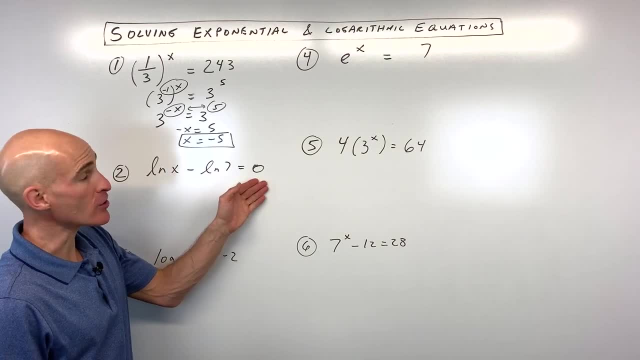 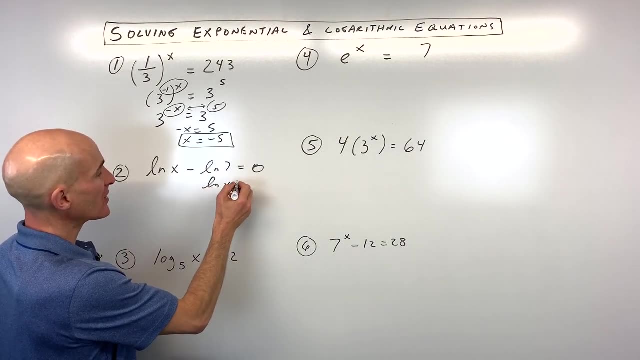 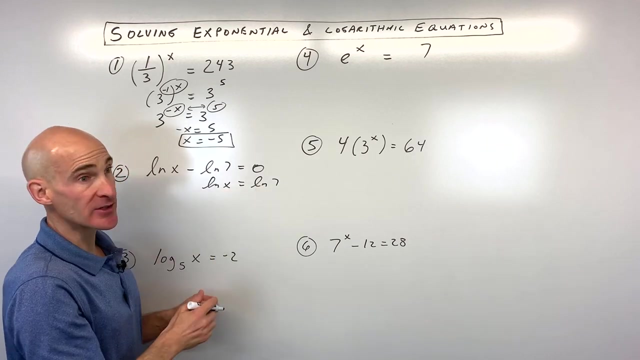 log equation. we have natural log of x minus natural log of seven equals zero. what I'm going to do on this one is I'm going to add natural log of seven to get it to the other side of the equation. So we have natural log of x. add this over so we get natural log of seven. And now what this is called is the one to one property of log. So as long as the bases are the same, which natural log? these are both base e. then what we can do is we can set these arguments equal to one another And we have x equals seven. Now one thing you want to pay attention to is that when you get your answer, when you're 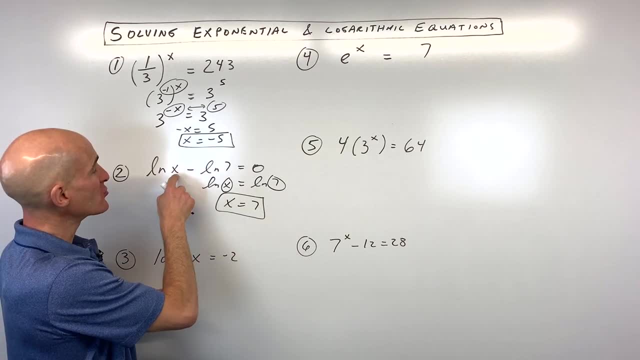 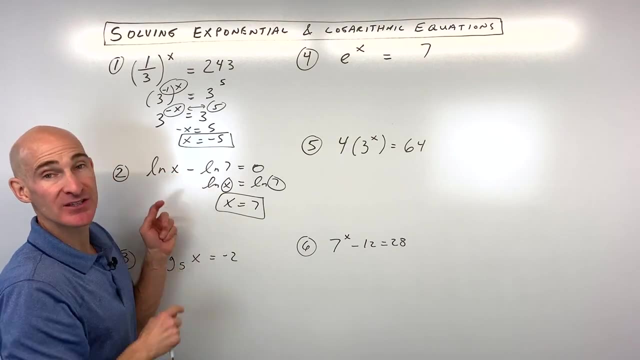 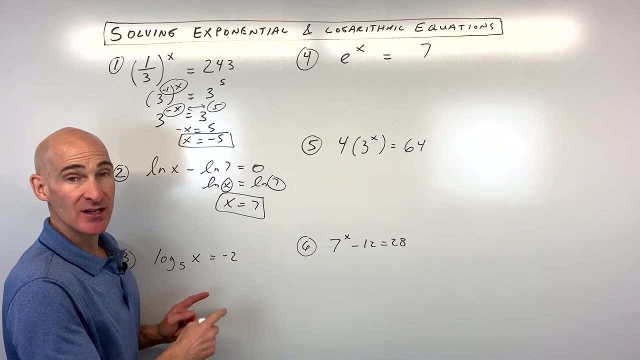 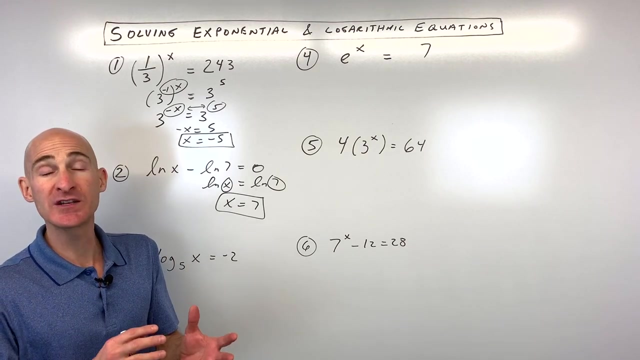 solving these log equations, you want to just put it back in and make sure that you're not taking the log or the natural log of a negative quantity or zero. So this whole thing here should be positive, Otherwise it's extraneous. So for number three, how would you do this? one log base five of x equals negative two. Well, an important skill that you want to master is knowing how to switch from the log form to the exponential form and vice versa. So the way I like to do this is I like to think of as logs and exponential functions as inverses of one and 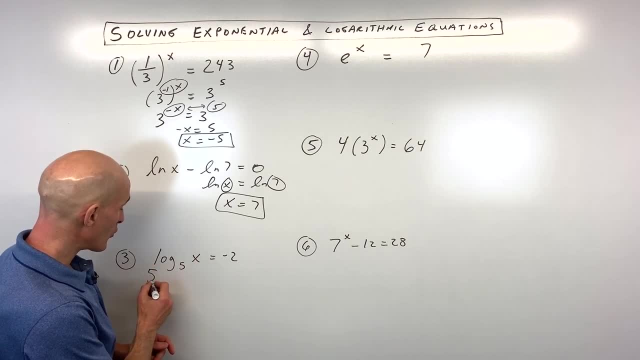 another. So if I'm taking the log, base five, what I'm going to do is I'm going to exponentiate, meaning I'm going to raise both sides using base five, Okay. And so now you can see these are inverses, So they cancel one another out, kind of like squaring and square rooting, or adding and subtracting their opposites. Okay, so they cancel each other. Five squared is 25.. But because it's a negative two, we're going to take the reciprocal, So that's one over 25.. And that's our final result. Now, remember what I mentioned about logs. you want to take that and put it back in? Yeah, we're not taking the 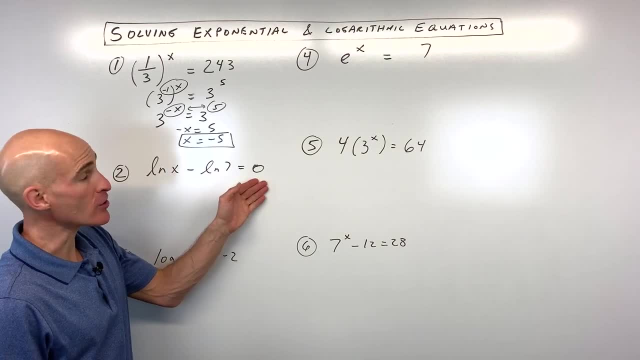 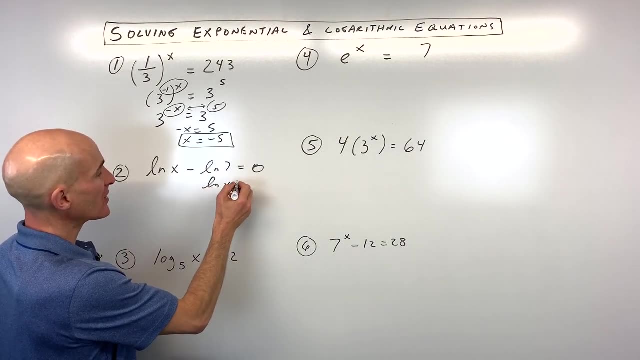 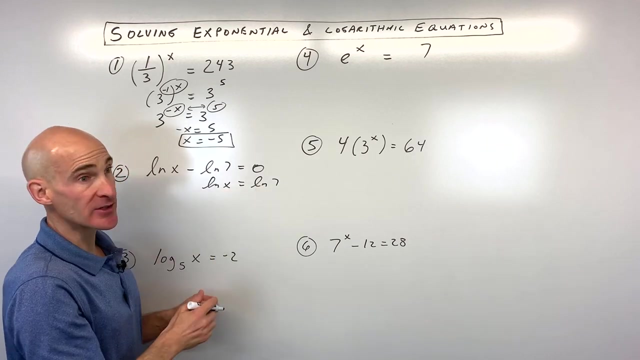 log equation. we have natural log of x minus natural log of seven equals zero. what I'm going to do on this one is I'm going to add natural log of seven to get it to the other side of the equation. So we have natural log of x. add this over so we get natural log of seven. And now what this is called is the one to one property of log. So as long as the bases are the same, which natural log? these are both base e. then what we can do is we can set these arguments equal to one another And we have x equals seven. Now one thing you want to pay attention to is that when you get your answer, when you're 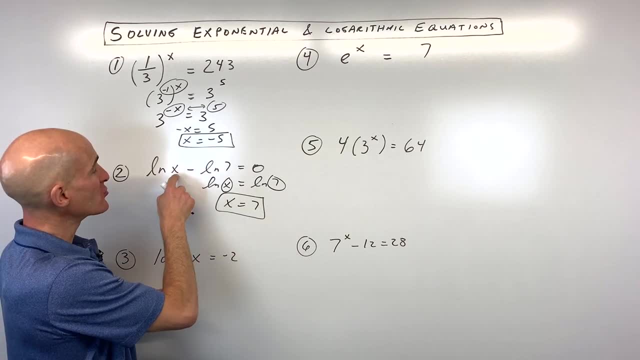 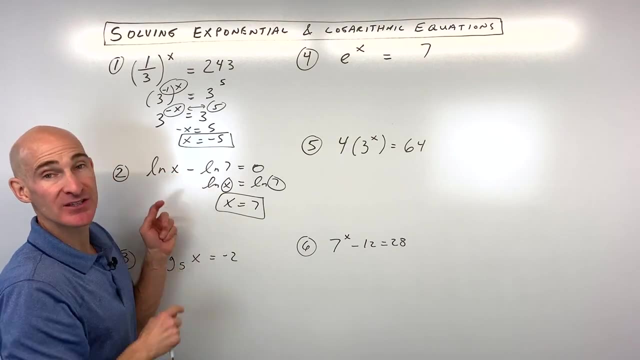 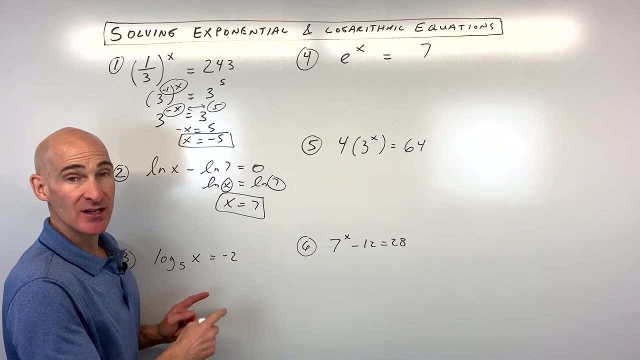 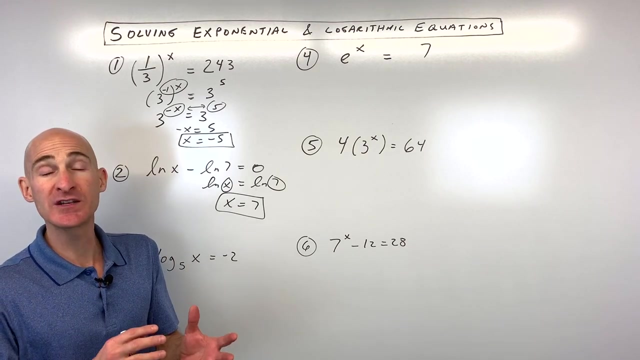 solving these log equations, you want to just put it back in and make sure that you're not taking the log or the natural log of a negative quantity or zero. So this whole thing here should be positive, Otherwise it's extraneous. So for number three, how would you do this? one log base five of x equals negative two. Well, an important skill that you want to master is knowing how to switch from the log form to the exponential form and vice versa. So the way I like to do this is I like to think of as logs and exponential functions as inverses of one and 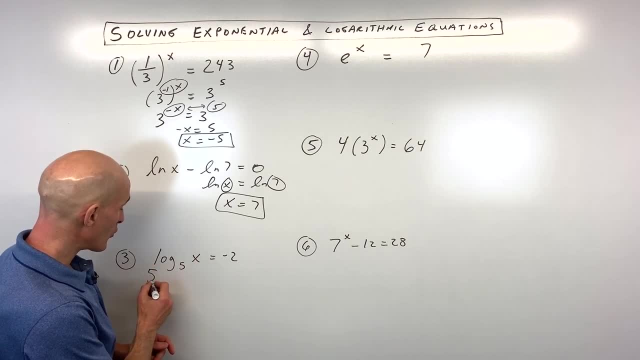 another. So if I'm taking the log, base five, what I'm going to do is I'm going to exponentiate, meaning I'm going to raise both sides using base five, Okay. And so now you can see these are inverses, So they cancel one another out, kind of like squaring and square rooting, or adding and subtracting their opposites. Okay, so they cancel each other. Five squared is 25.. But because it's a negative two, we're going to take the reciprocal, So that's one over 25.. And that's our final result. Now, remember what I mentioned about logs. you want to take that and put it back in? Yeah, we're not taking the 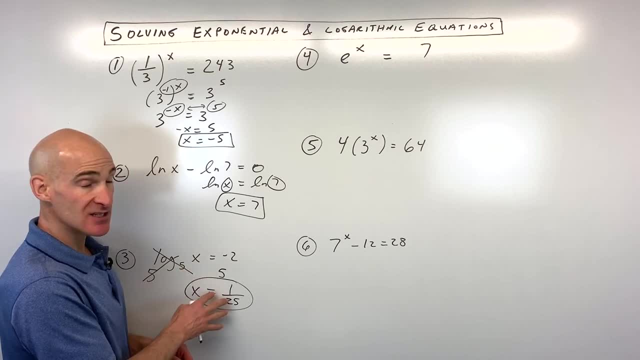 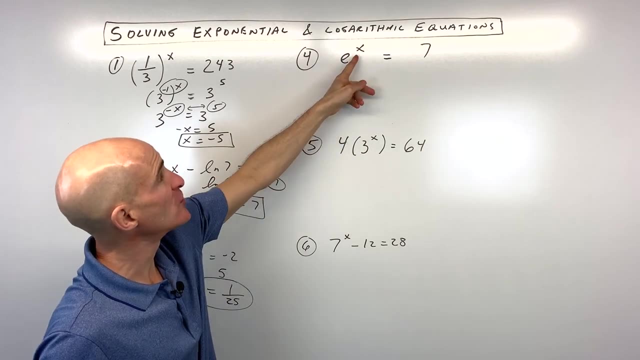 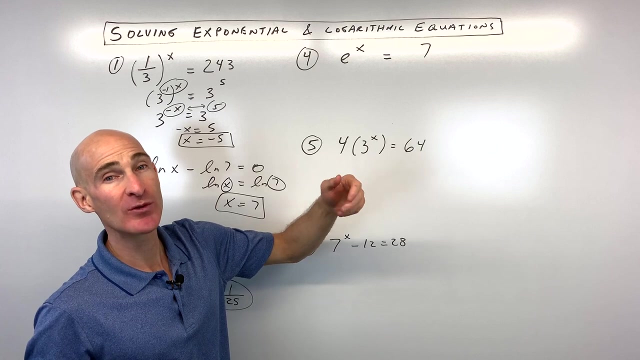 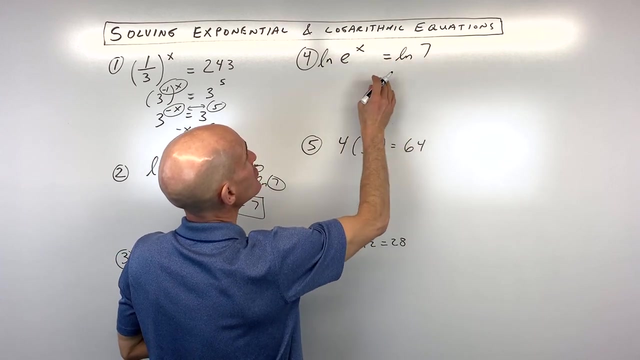 log of, you know, a negative or zero quantity. So that means this is perfectly good. So for number four we've got e to the x equals seven. So here what we want to do is because that variables in the exponent position is we want to bring it down from there By doing the inverse, okay, of exponentiating. we want to take the log, or the natural log of both sides of this equation. So I'm just going to write natural log, natural log. I'm doing it to both sides to keep it balanced. Remember, natural log is really like log base e. 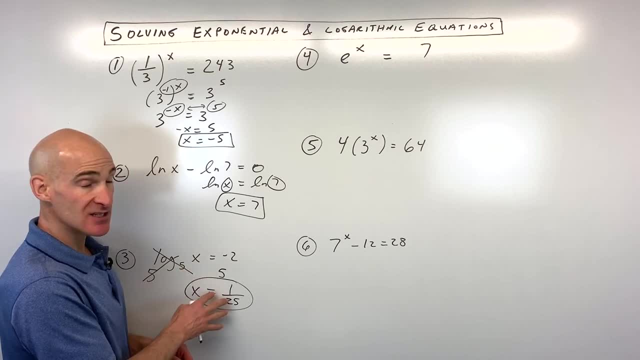 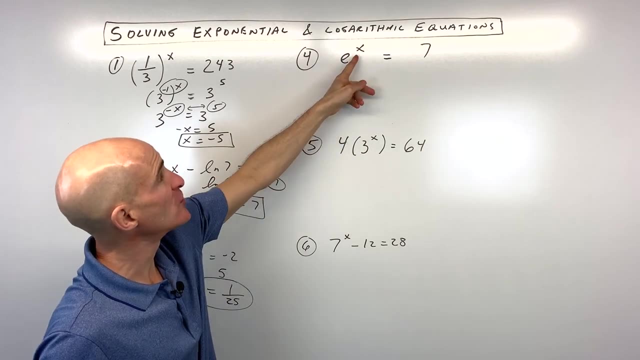 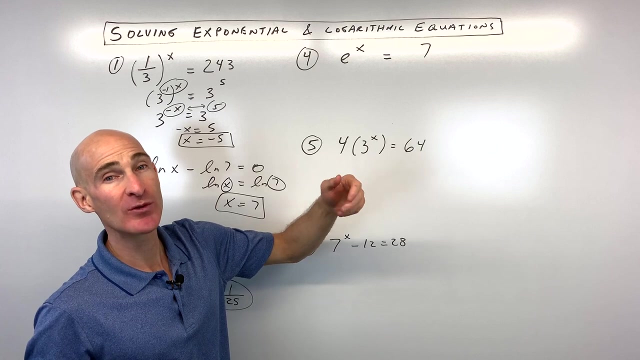 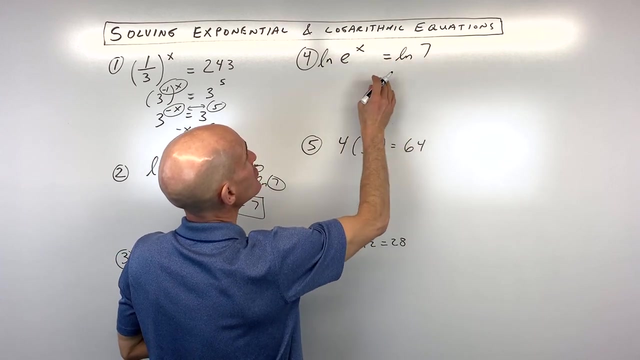 log of, you know, a negative or zero quantity. So that means this is perfectly good. So for number four we've got e to the x equals seven. So here what we want to do is because that variables in the exponent position is we want to bring it down from there By doing the inverse, okay, of exponentiating. we want to take the log, or the natural log of both sides of this equation. So I'm just going to write natural log, natural log. I'm doing it to both sides to keep it balanced. Remember, natural log is really like log base e. 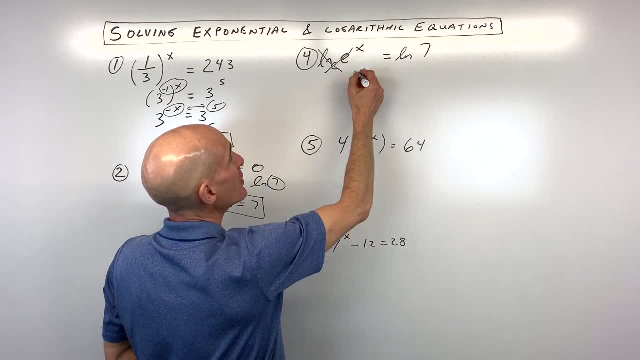 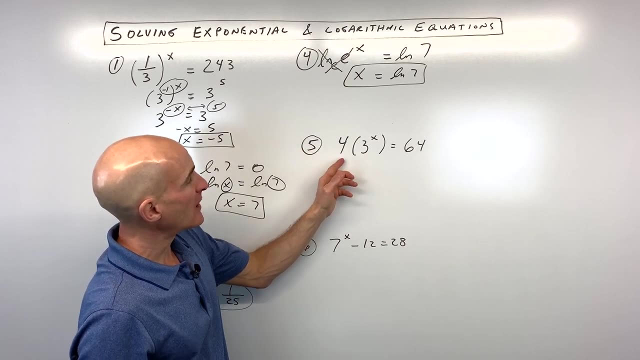 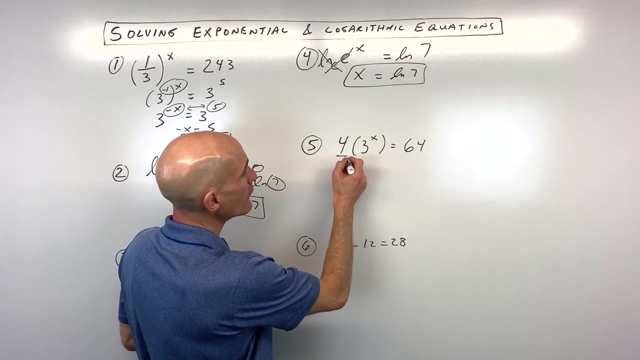 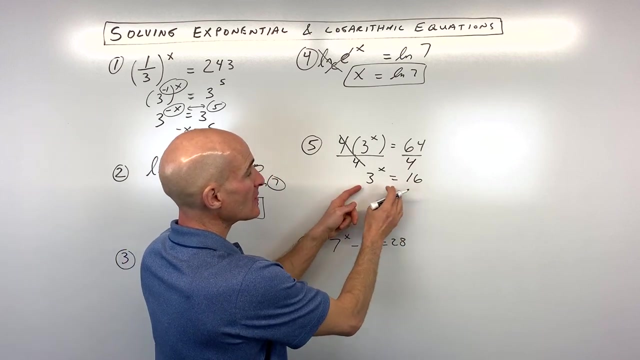 These are inverses of one another, So they cancel each other out and you have x equals natural log of seven. that's your final result. Okay, for number five, this one. okay. what we want to do is we want to work from the outside in towards this variable x. we're trying to get the variable by itself, So instead of multiplying by four, let's divide both sides by four. Okay, and now we have three to the x equals 16.. We can't get the bases the same here, okay, because three to what power is 16.. But what we want to do is: 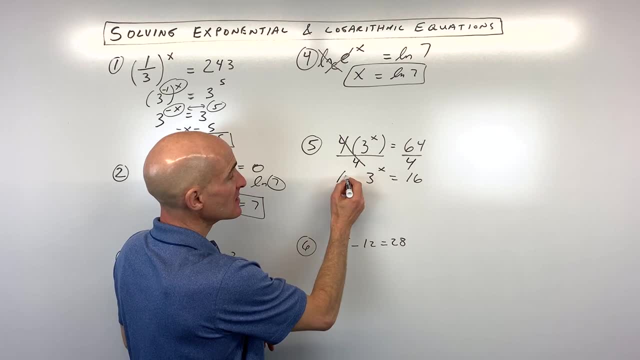 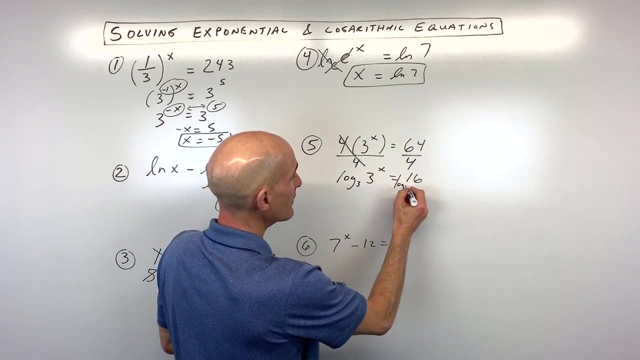 is. we want to say: well, what's the opposite of exponentiating? Let's take the logarithm. We just want to make sure that these bases are the same. So I'm going to take log base 3 of this side and log base 3 of the other side to keep it balanced right. So these are inverses, and so we have x. 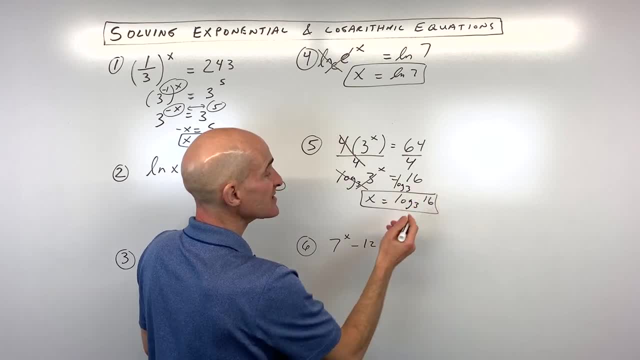 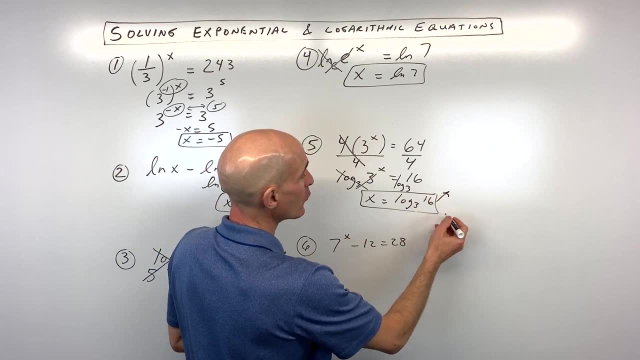 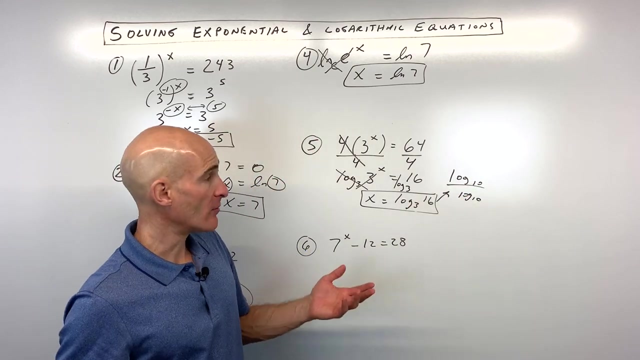 equals log base 3 of 16.. This is an exact answer. Now, if your calculator doesn't allow you to change the base, okay, what you can do is you can use the change of base formula, which looks like this: Log base 10.. You can pick any base, like natural log log base 5,. 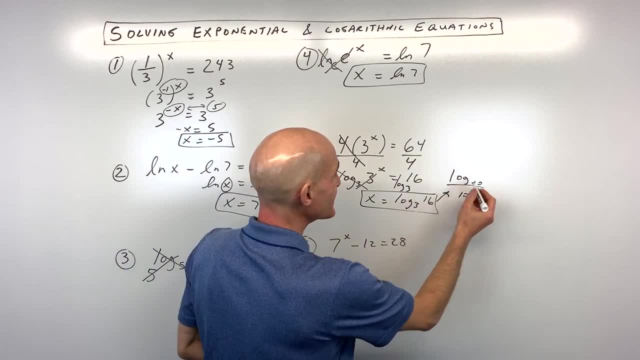 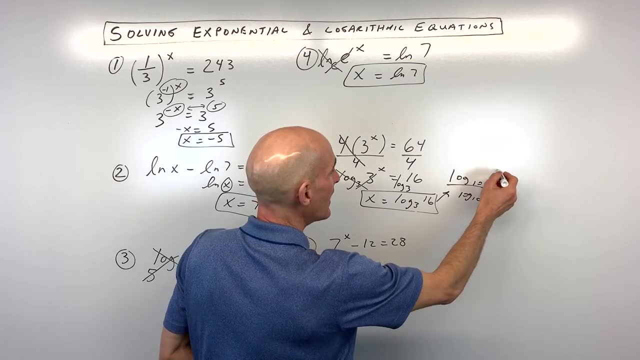 but here on most calculators you have log base 10 or the common log. 16 goes in the numerator, 3 goes in the denominator. So it's easy to remember because the 3 is a little bit lower right 16 is a little bit higher. That's an easy way to remember it. That's your change of base. 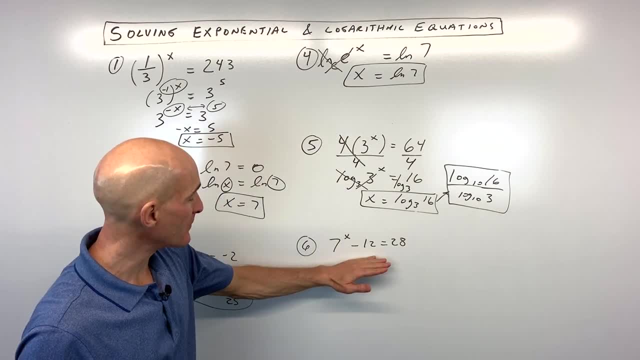 These are equivalent. You can get a decimal approximation on your calculator For number 6, we want to solve for x here. So again like this one, we want to work from the outside, We want to work from the inside. We want to work from the outside, We want to work from. 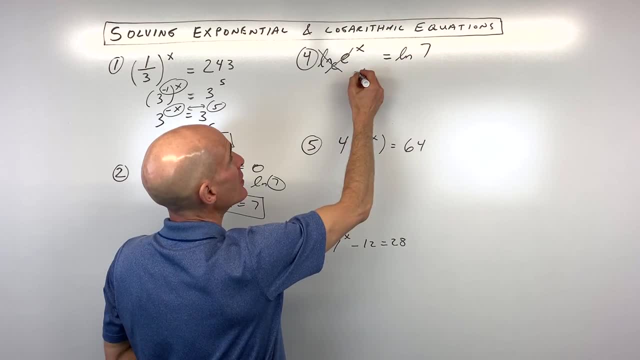 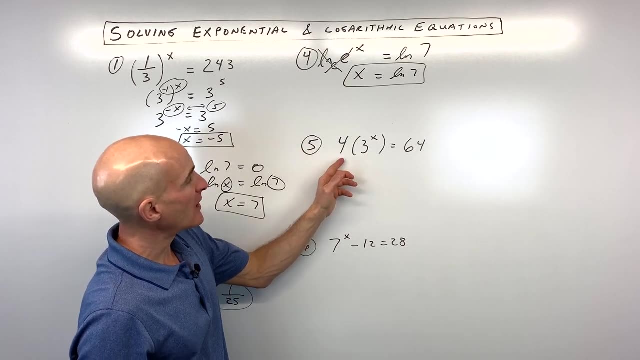 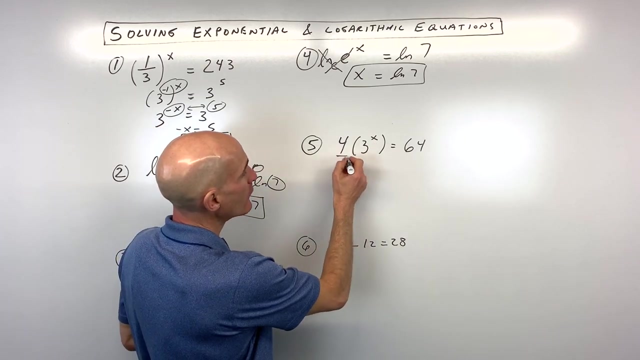 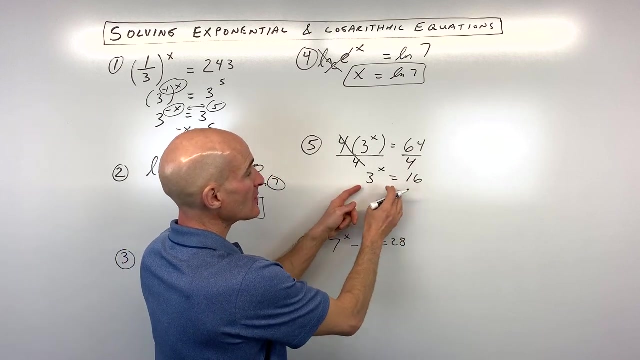 These are inverses of one another, So they cancel each other out and you have x equals natural log of seven. That's your final result. Okay, for number five, this one. okay. what we want to do is we want to work from the outside in towards this variable x. we're trying to get the variable by itself, So instead of multiplying by four, let's divide both sides by four. Okay, and now we have three to the x equals 16.. We can't get the bases the same here. Okay, because three to what power is 16.. But what we want to do, 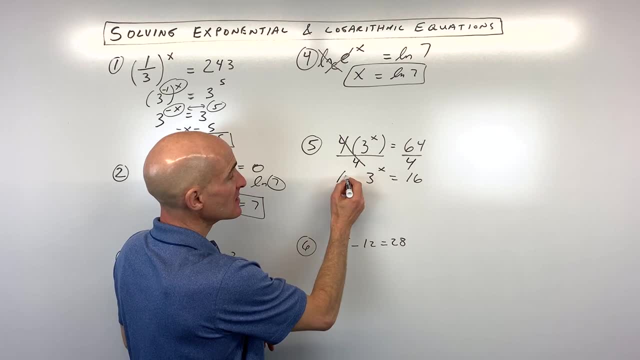 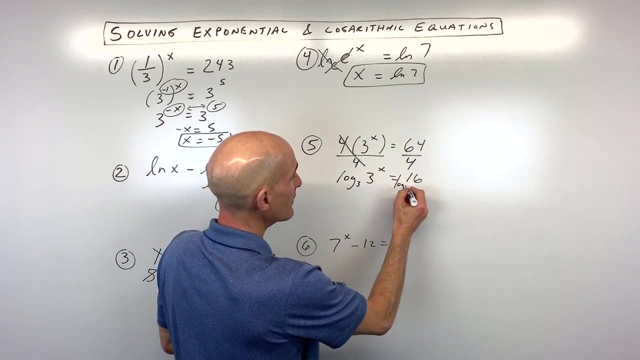 is. we want to say: well, what's the opposite of exponentiating? Let's take the logarithm. We just want to make sure that these bases are the same. So I'm going to take log base 3 of this side and log base 3 of the other side to keep it balanced right. So these are inverses, and so we have x. 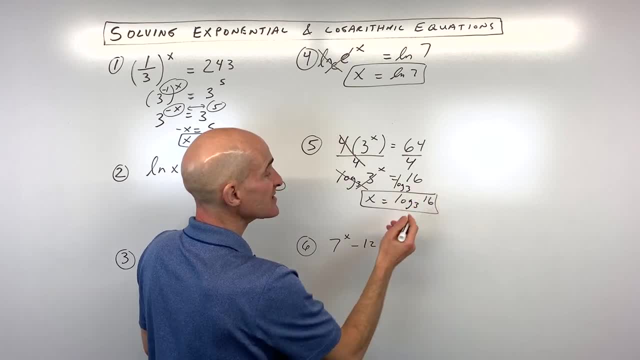 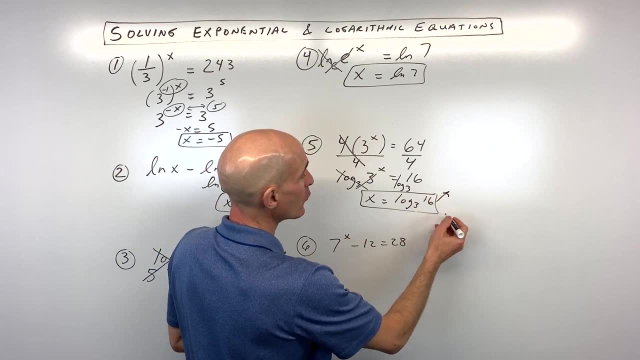 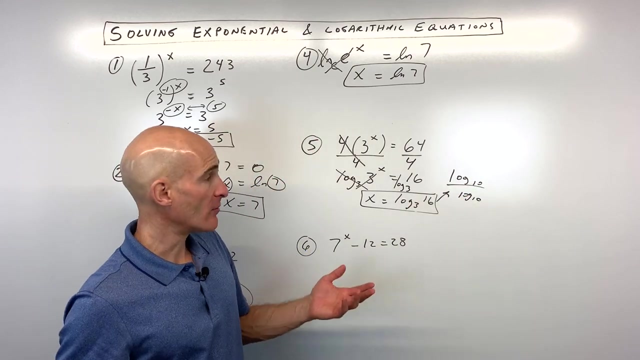 equals log base 3 of 16.. This is an exact answer. Now, if your calculator doesn't allow you to change the base, okay, what you can do is you can use the change of base formula, which looks like this: Log base 10.. You can pick any base, like natural log log base 5,. 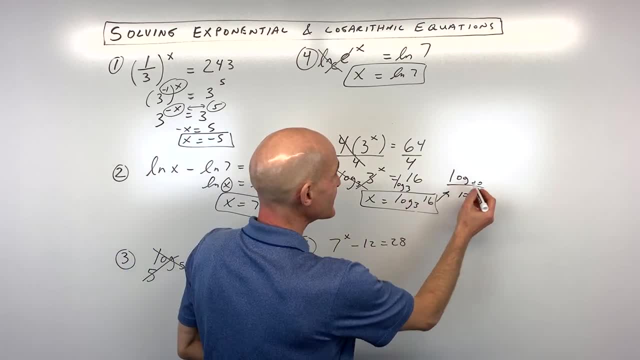 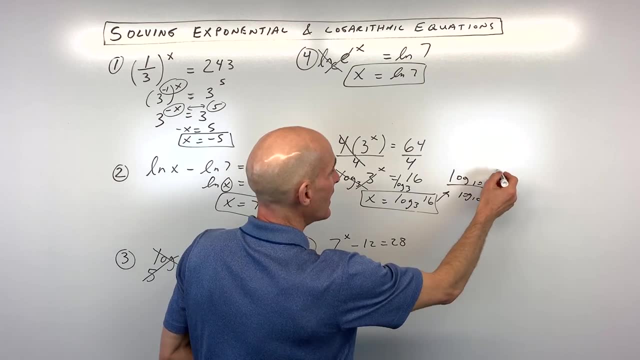 but here on most calculators you have log base 10 or the common log. 16 goes in the numerator, 3 goes in the denominator. So it's easy to remember because the 3 is a little bit lower right 16 is a little bit higher. That's an easy way to remember it. That's your change of base. 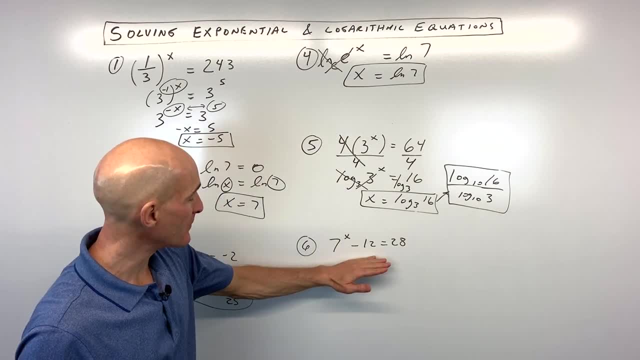 These are equivalent. You can get a decimal approximation on your calculator For number 6, we want to solve for x here. So again like this one, we want to work from the outside, We want to work from the inside. We want to work from the outside, We want to work from. 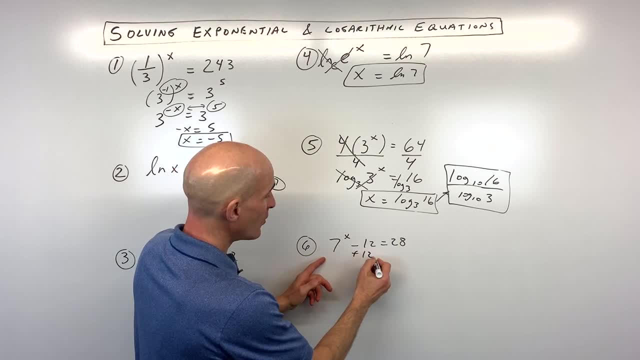 the outside, We want to work from the inside, We want to work from the outside, We want to work from the inside in towards that variable. So what I'm going to do is I'm going to add 12 to both sides, So that's going to give us 7 to the x equals 40. Well, we can't get the bases the same. 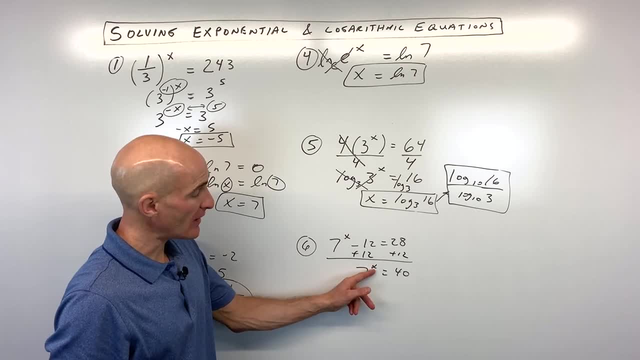 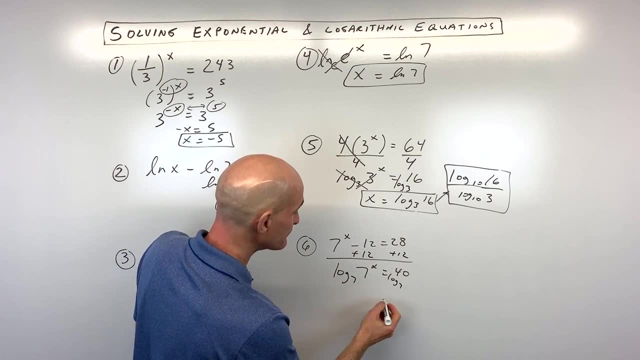 okay, like we did in that first problem. But what we can do is we can say: well, that variable's in the exponent position, So let's go ahead and do the inverse. Let's take the log base 7 of both sides right? So those are inverses or opposites, And you can see we just ended up with x equals. 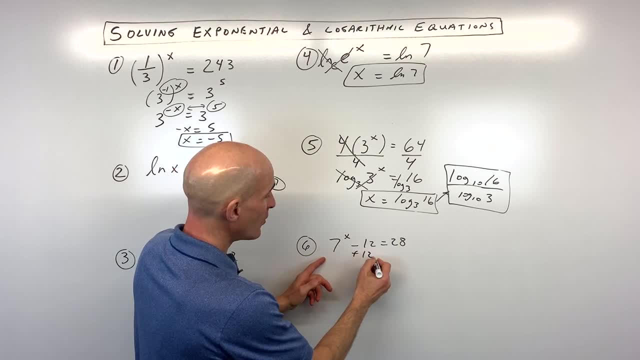 the outside, We want to work from the inside, We want to work from the outside, We want to work from the inside in towards that variable. So what I'm going to do is I'm going to add 12 to both sides, So that's going to give us 7 to the x equals 40. Well, we can't get the bases the same. 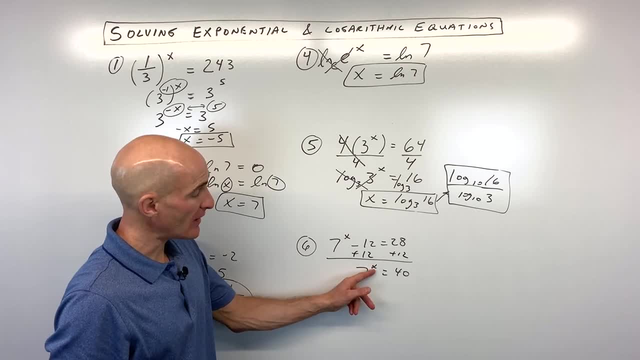 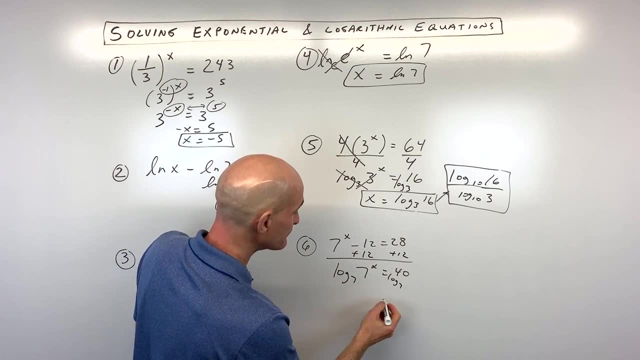 okay, like we did in that first problem. But what we can do is we can say: well, that variable's in the exponent position, So let's go ahead and do the inverse. Let's take the log base 7 of both sides right? So those are inverses or opposites, And you can see we just ended up with x equals. 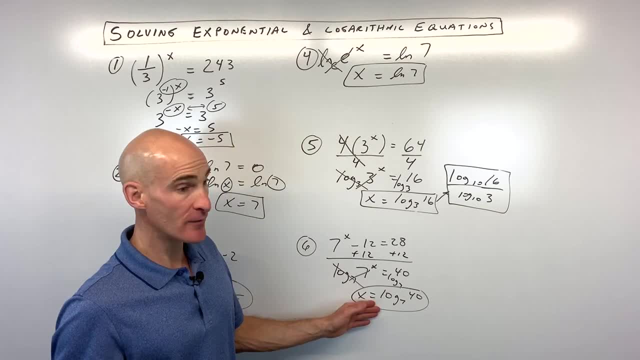 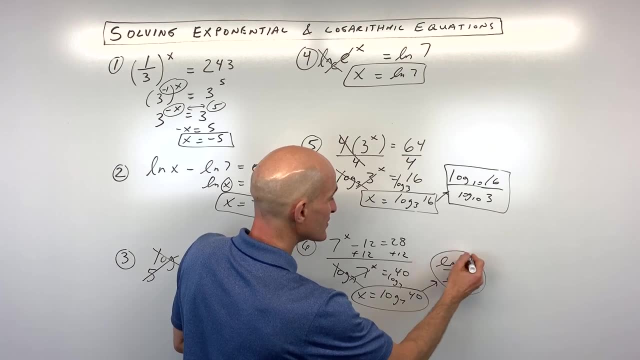 log base 7 of 40.. If you want to use the change of base formula, we can do that Here. I'll use the natural logs for this one, Natural log of 40 over natural log of 7.. You can put this in your calculator and get a decimal approximation. Okay, we're getting a little bit. 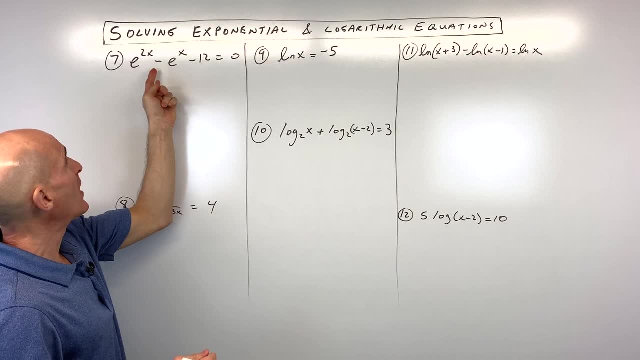 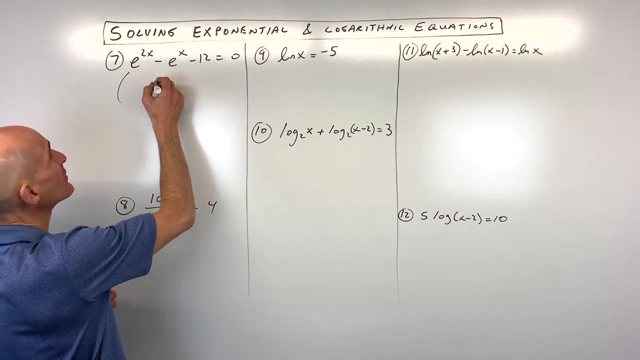 more challenging here. now Number 7, we've got e to the 2x minus e to the x minus 12 equals 0. So the technique you want to use on this particular problem is to factor into two binomials. So here: 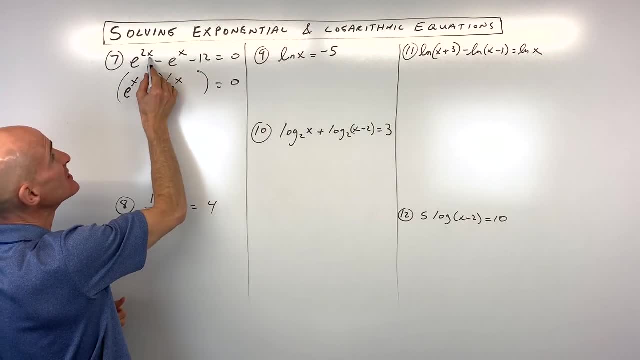 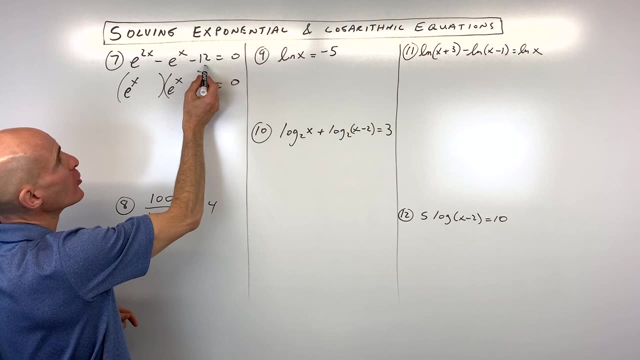 we can see: e to the x, times e to the x equals e to the 2x, Because, remember, when you multiply you add the exponent, So x plus x equals 2x. And here we say what multiplies to negative 12, but adds to negative. 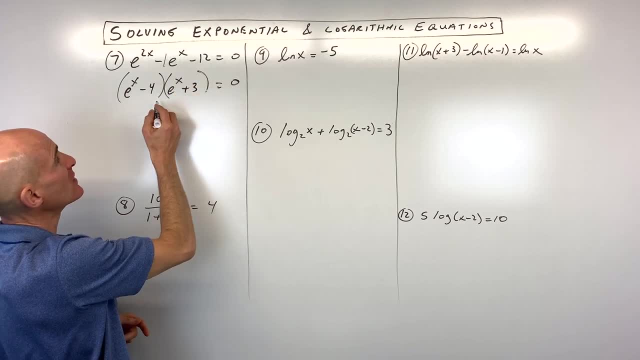 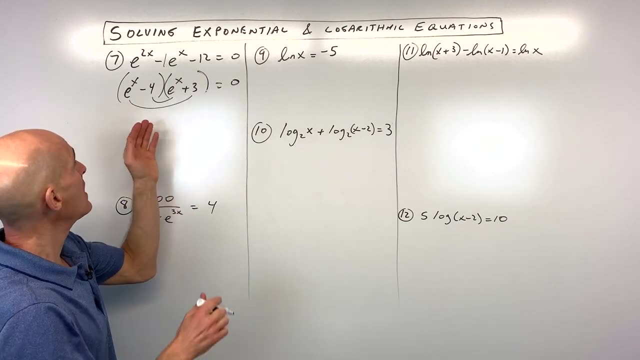 1, that's going to be negative 4 and positive 3.. And you can see that negative 4 e to the x and positive 3 e to the x equals the middle term, which is negative 1 e to the x. Now that we have, 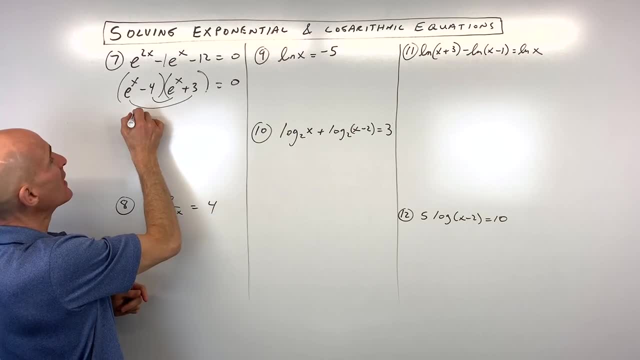 it factored, we can set each of these factors equal to 0. So we have e to the x minus 4 equals 0, and e to the x plus 3 equals 0.. If we add 4 to both sides, we have e to the x equals 4,. 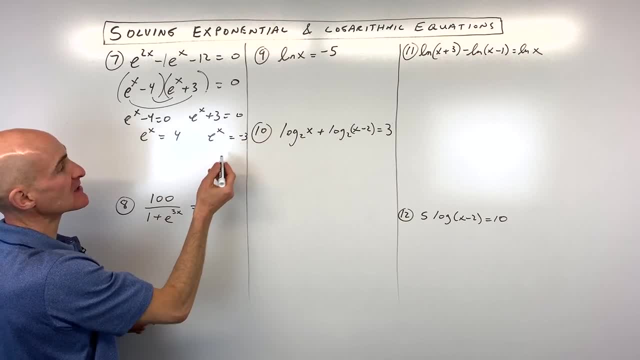 and if we subtract 3 from both sides, we have e to the x equals negative 3.. Now what I'm going to do? because that variable is in the exponent position, I'm going to do the inverse. I'm going to take the log, or the natural log, in this case, of both sides. Remember, natural log is log base. 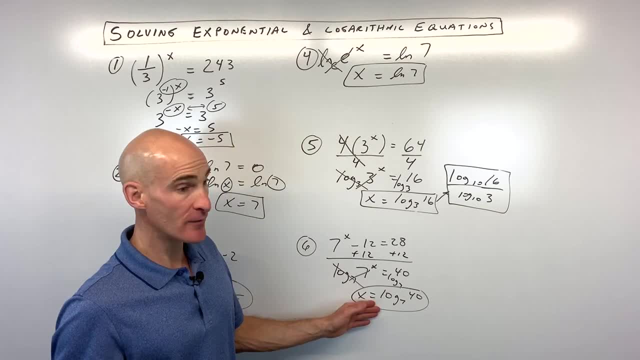 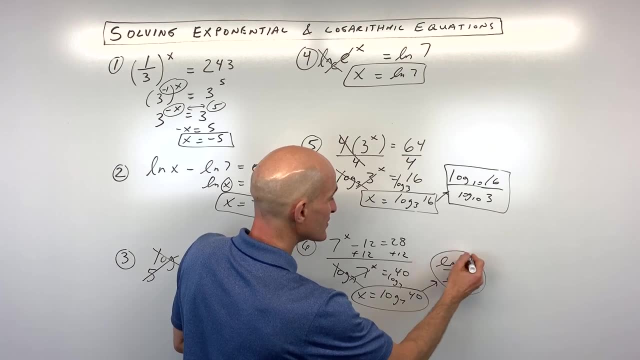 log base 7 of 40.. If you want to use the change of base formula, we can do that Here. I'll use the natural logs for this one, Natural log of 40 over natural log of 7.. You can put this in your calculator and get a decimal approximation. Okay, we're getting a little bit. 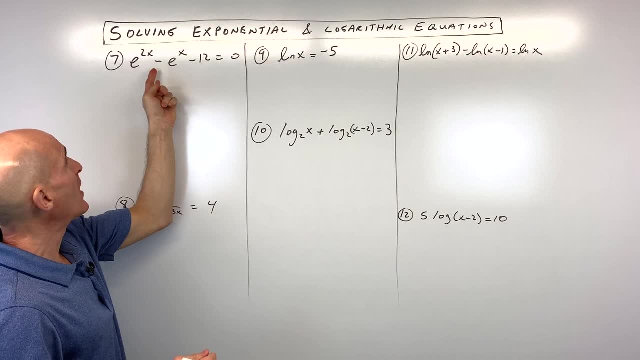 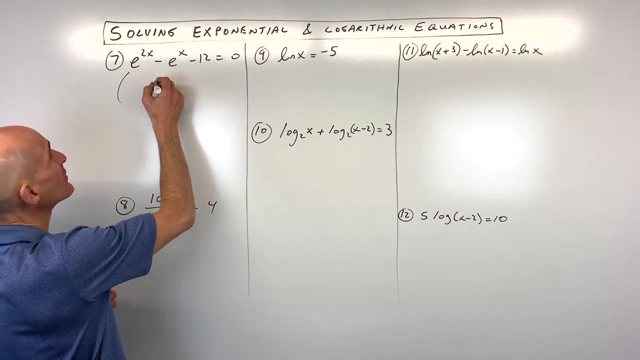 more challenging here. now Number 7, we've got e to the 2x minus e to the x minus 12 equals 0. So the technique you want to use on this particular problem is to factor into two binomials. So here: 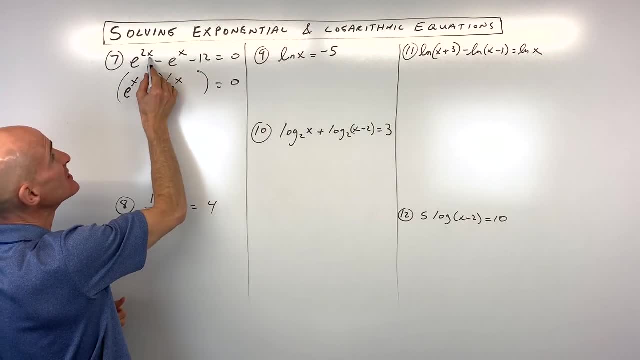 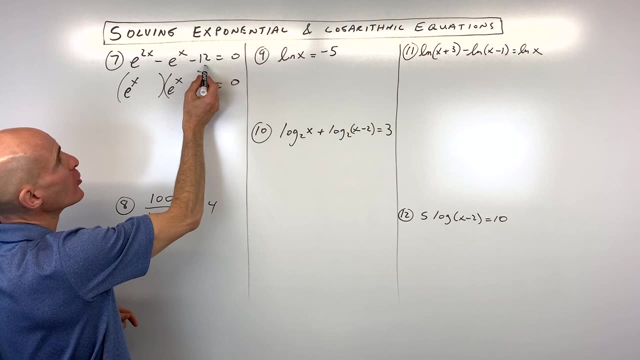 we can see: e to the x, times e to the x equals e to the 2x, Because, remember, when you multiply you add the exponent, So x plus x equals 2x. And here we say what multiplies to negative 12, but adds to negative. 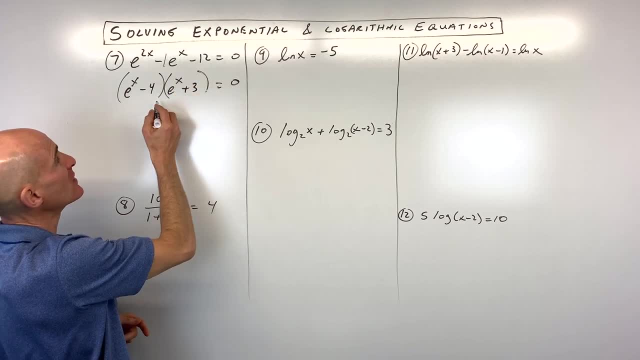 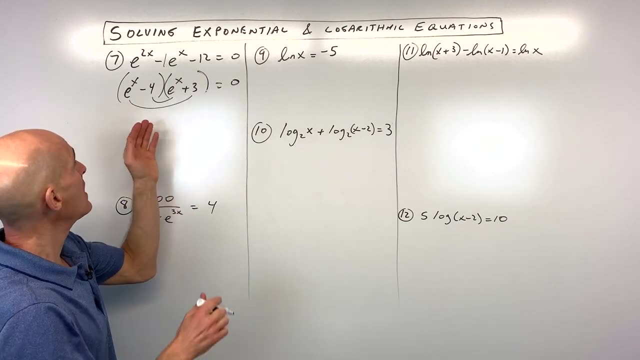 1, that's going to be negative 4 and positive 3.. And you can see that negative 4 e to the x and positive 3 e to the x equals the middle term, which is negative 1 e to the x. Now that we have, 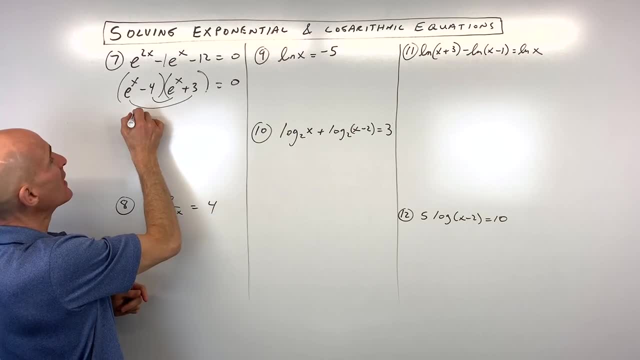 it factored, we can set each of these factors equal to 0. So we have e to the x minus 4 equals 0, and e to the x plus 3 equals 0.. If we add 4 to both sides, we have e to the x equals 4,. 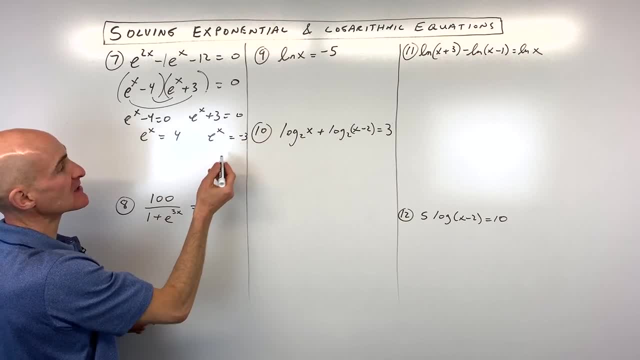 and if we subtract 3 from both sides, we have e to the x equals negative 3.. Now what I'm going to do? because that variable is in the exponent position, I'm going to do the inverse. I'm going to take the log, or the natural log, in this case, of both sides. Remember, natural log is log base. 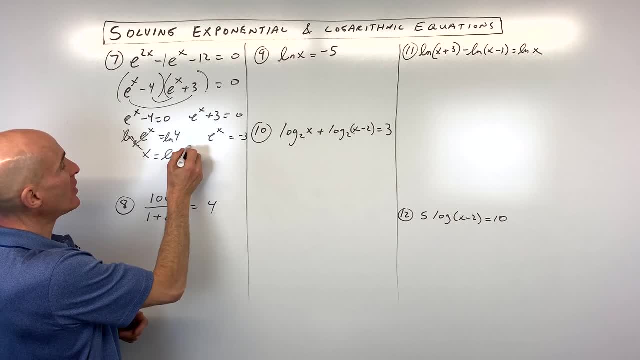 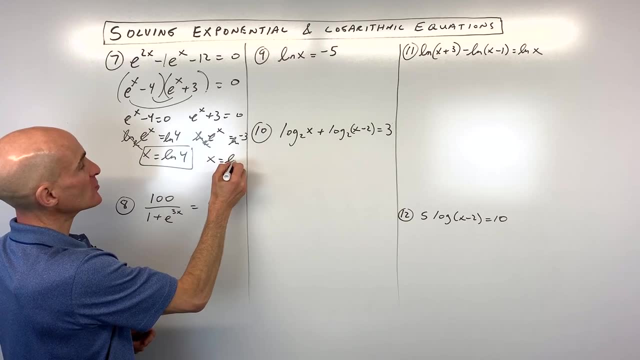 e. So these are inverses. So we get x equals natural log of 4.. Here, if we take the natural log of both sides, these are inverses. So we get x equals natural log of negative 3.. But remember: 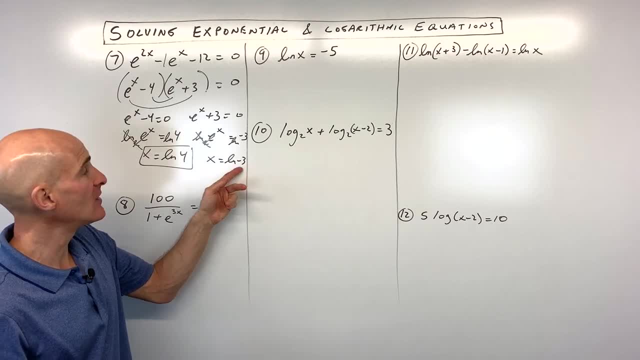 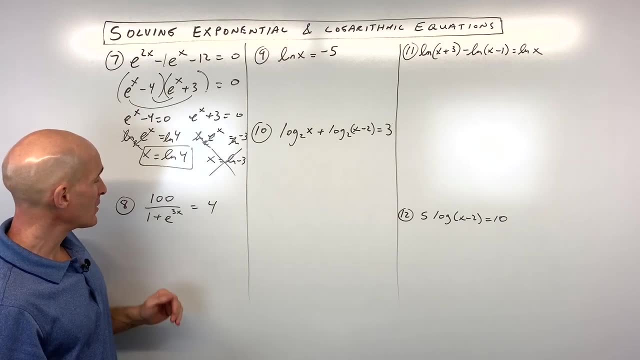 we talked about earlier. you can't take the log of both sides, So we get x equals natural log of negative 3.. So this is extraneous. We're just going to cross that out. It's just going to be natural log of 4.. Okay, for number 8,. what do you think for this one, A little bit more challenging. 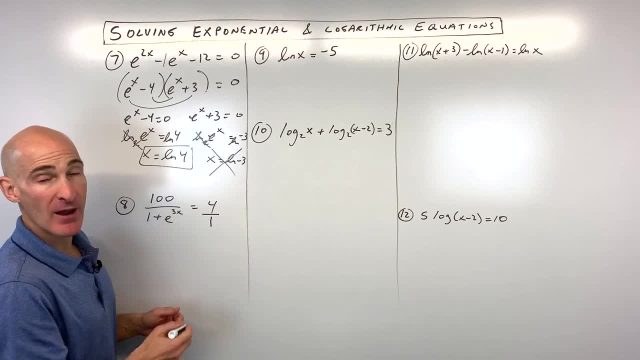 What I would probably do on this one is think of this as 4 divided by 1. And when you have a fraction equal to a fraction or a ratio equal to a ratio, this forms a proportion And you can cross, multiply on the diagonal. So 4 times 1, plus e to the 3x, I'm going to distribute to 4.. So 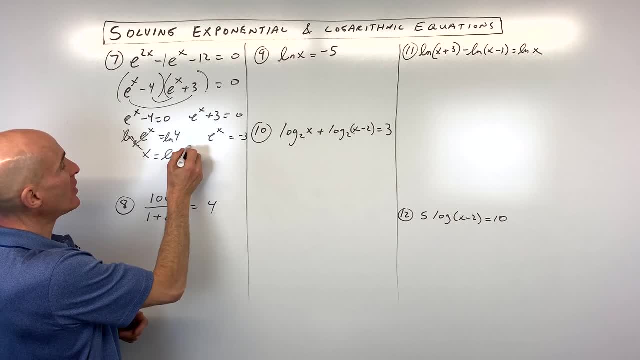 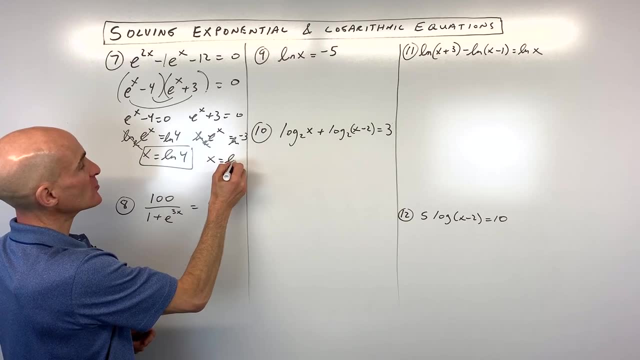 e. So these are inverses. So we get x equals natural log of 4.. Here, if we take the natural log of both sides, these are inverses. So we get x equals natural log of negative 3.. But remember: 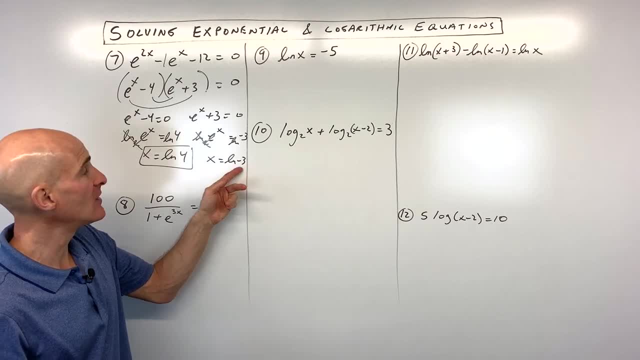 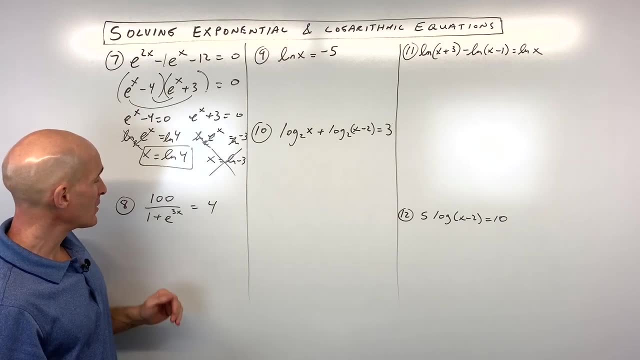 we talked about earlier. you can't take the log of both sides, So we get x equals natural log of negative 3.. So this is extraneous. We're just going to cross that out. It's just going to be natural log of 4.. Okay, for number 8,. what do you think for this one, A little bit more challenging. 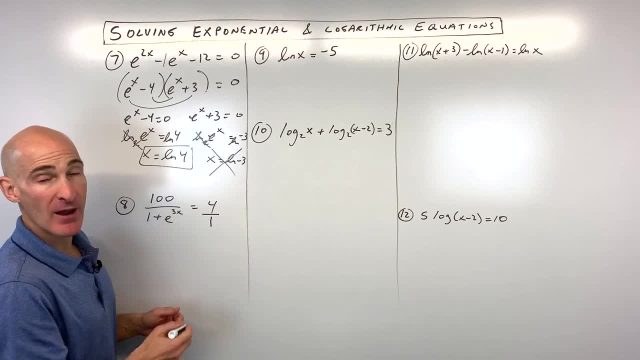 What I would probably do on this one is think of this as 4 divided by 1. And when you have a fraction equal to a fraction or a ratio equal to a ratio, this forms a proportion And you can cross, multiply on the diagonal. So 4 times 1, plus e to the 3x, I'm going to distribute to 4.. So 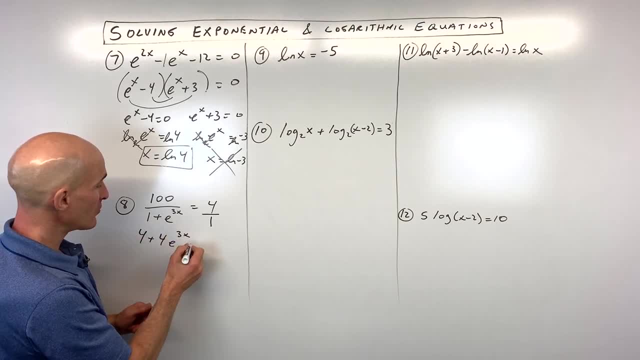 that's going to be 4.. Plus 4e to the 3x equals 100 times 1, which is 100.. Let's subtract 4 from both sides, So that's 4e to the 3x equals 96.. Let's divide both sides by 4.. So e to the 3x equals, let's see what would. 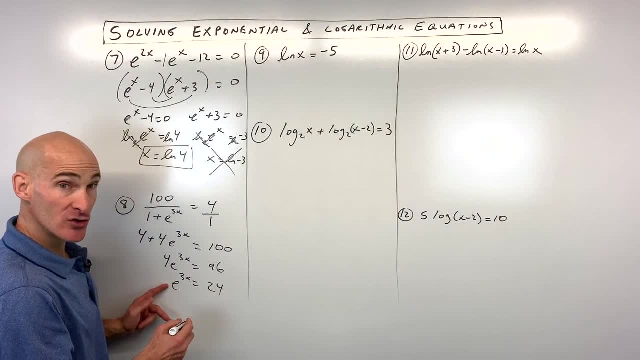 that be 24.. Okay, good, And then we just have to do the inverse. now, Instead of exponentiating, we're going to take the log of both sides, or, in this case, the natural log, because this is base e, Those are inverses, And we have 3x equals. 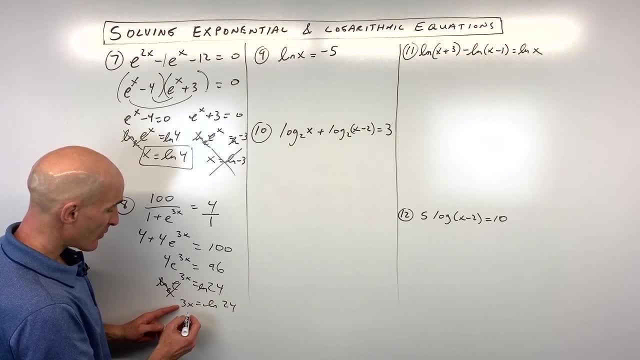 natural log of 24.. Divide both sides by 3, or you could multiply both sides by 1- 3rd to get x by itself. So that's 1: 3rd natural log of 24.. And you got it. Now, if you want to get a little bit, 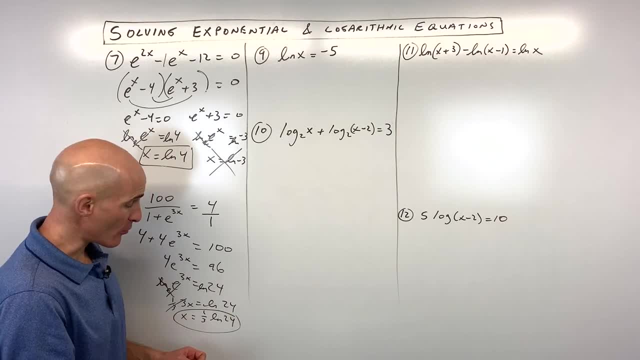 fancy, you could bring up this 1, 3rd as a power. That's the power property of logs. And remember the 1, 3rd is like the cube root. So another option here would be to write this as natural log of cube root of 24.. Okay, for number 9, we have a little simpler one. Natural log of x equals: 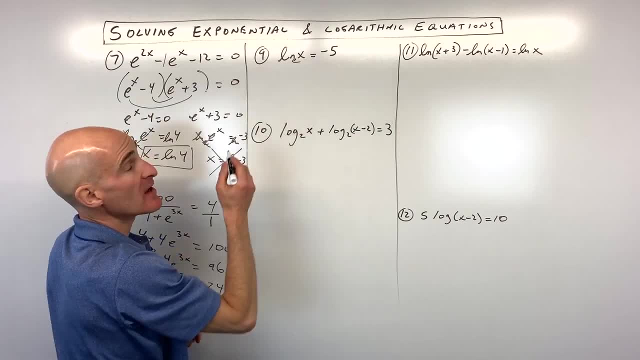 negative 5. And we're going to divide both sides by 3.. So that's 1. 3rd natural log of 24.. And we're going to do that. Remember, this is understood to be base e. So what we're going to do is we're. 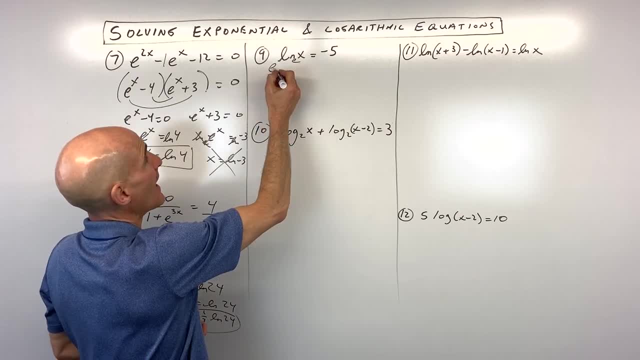 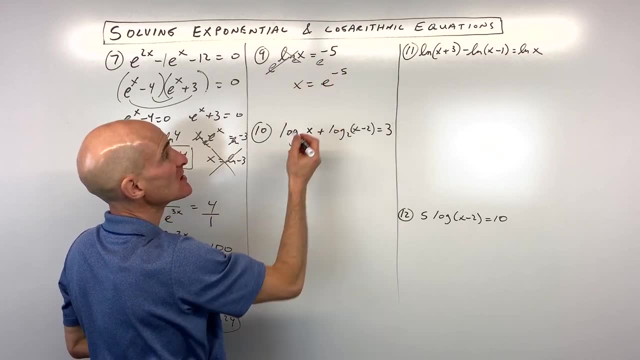 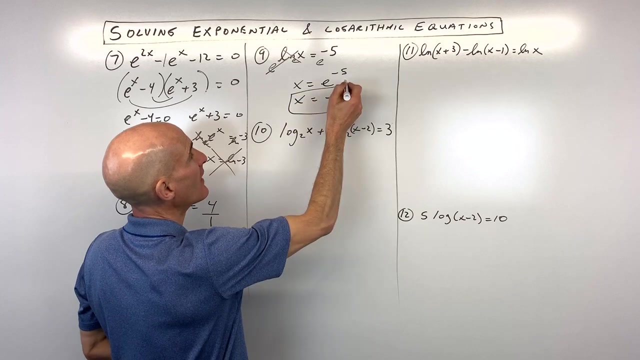 going to do the inverse of natural log, which is to exponentiate both sides using base e. So these are inverses. We get x by itself, So we have x equals e to the negative 5th. Or, because this is a negative exponent, we can take the reciprocal and write this as 1 over e to the positive 5.. 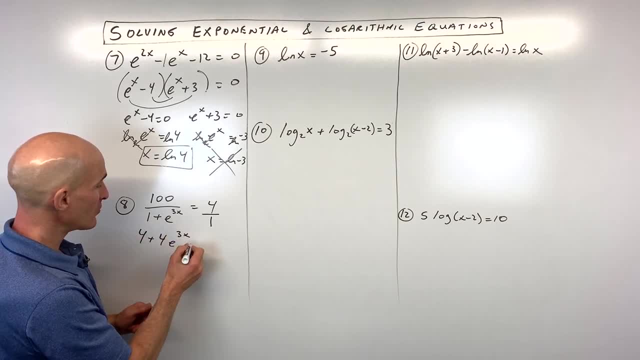 that's going to be 4.. Plus 4e to the 3x equals 100 times 1, which is 100.. Let's subtract 4 from both sides, So that's 4e to the 3x equals 96.. Let's divide both sides by 4.. So e to the 3x equals, let's see what would. 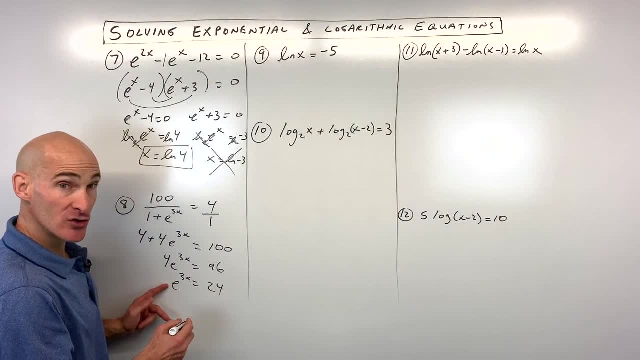 that be 24.. Okay, good, And then we just have to do the inverse. now, Instead of exponentiating, we're going to take the log of both sides, or, in this case, the natural log, because this is base e, Those are inverses, And we have 3x equals. 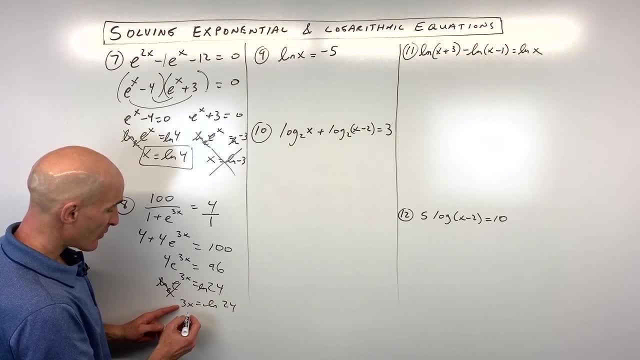 natural log of 24.. Divide both sides by 3, or you could multiply both sides by 1- 3rd to get x by itself. So that's 1: 3rd natural log of 24.. And you got it. Now, if you want to get a little bit, 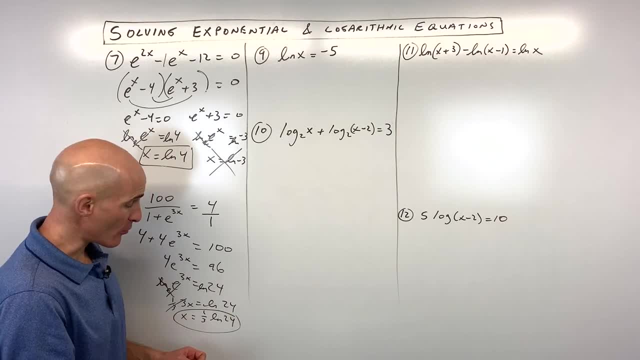 fancy, you could bring up this 1, 3rd as a power. That's the power property of logs. And remember the 1, 3rd is like the cube root. So another option here would be to write this as natural log of cube root of 24.. Okay, for number 9, we have a little simpler one. Natural log of x equals: 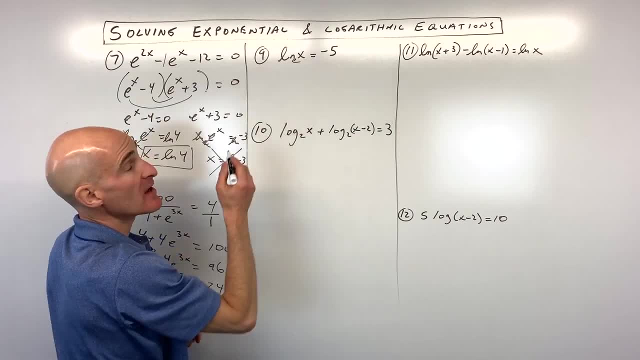 negative 5. And we're going to divide both sides by 3.. So that's 1. 3rd natural log of 24.. And we're going to do that. Remember, this is understood to be base e. So what we're going to do is we're. 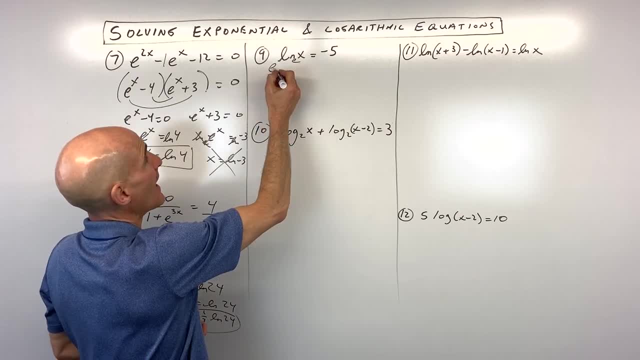 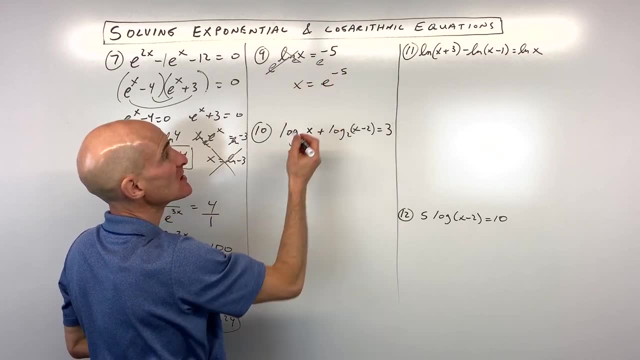 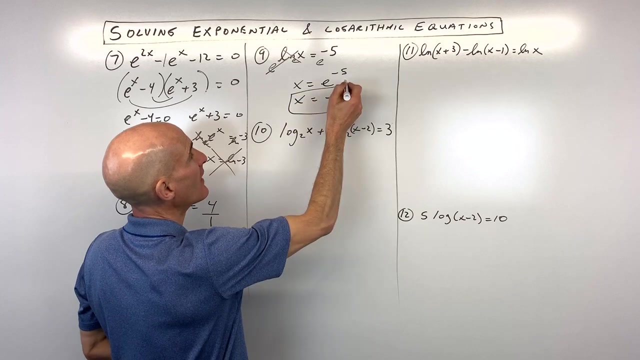 going to do the inverse of natural log, which is to exponentiate both sides using base e. So these are inverses. We get x by itself, So we have x equals e to the negative 5th. Or, because this is a negative exponent, we can take the reciprocal and write this as 1 over e to the positive 5.. 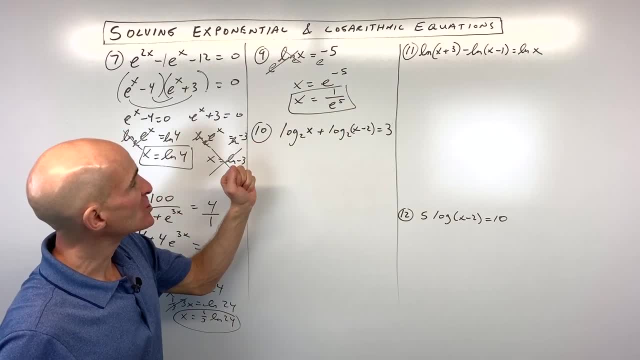 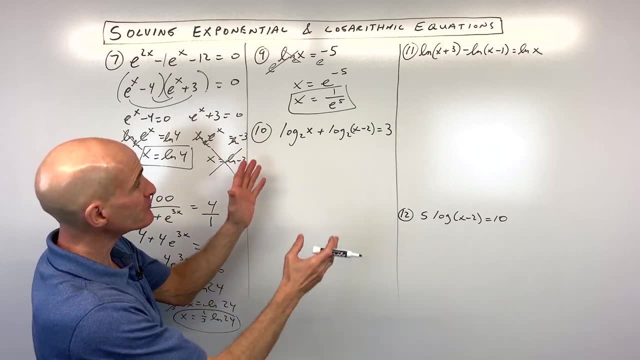 And that's your final result there. For number 10, a little bit more challenging, we've got log base 2 of x plus log base 2 of x, minus 2 equals 3.. What I'm going to do on this problem is use our condensing properties to condense this into. 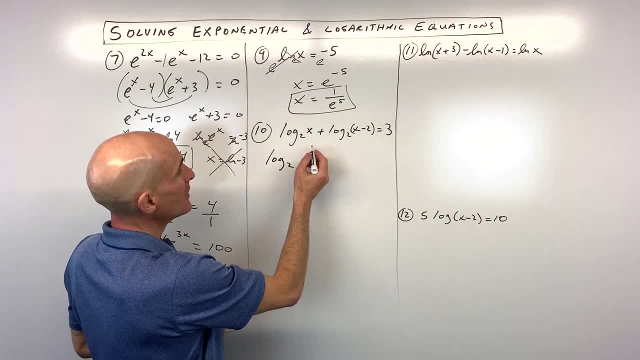 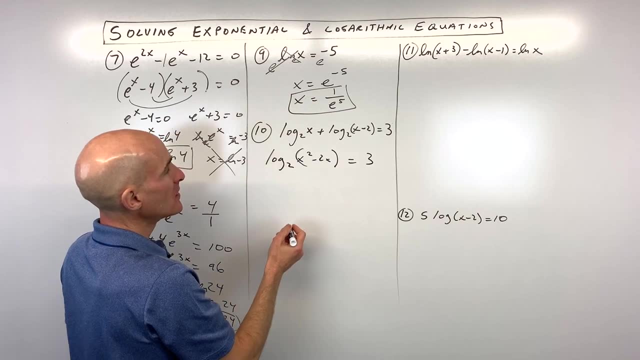 one log. So what we have is log base 2 of x times x minus 2, which comes out to x squared minus 2x equals 3.. So remember, when you add, you multiply. Now what we're going to do is we're going to. 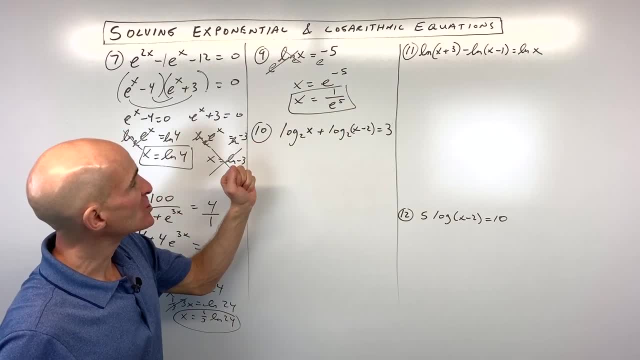 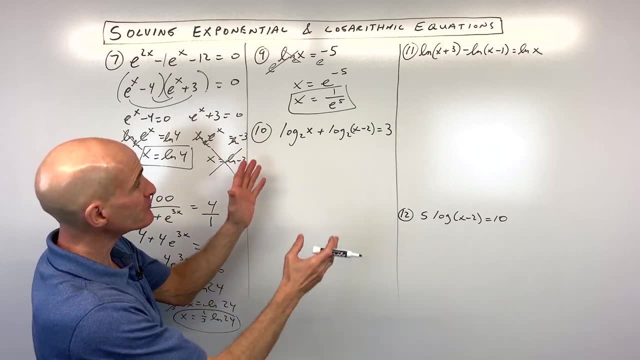 And that's your final result there. For number 10, a little bit more challenging, we've got log base 2 of x plus log base 2 of x, minus 2 equals 3.. What I'm going to do on this problem is use our condensing properties to condense this into. 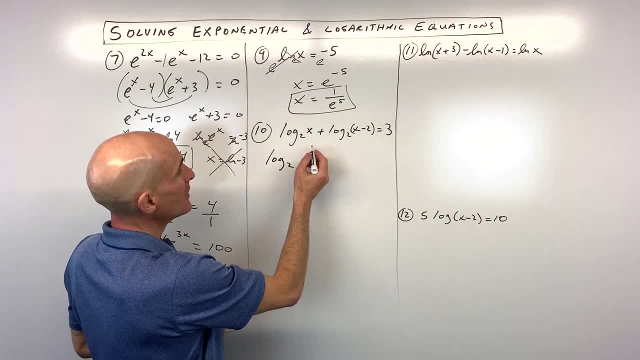 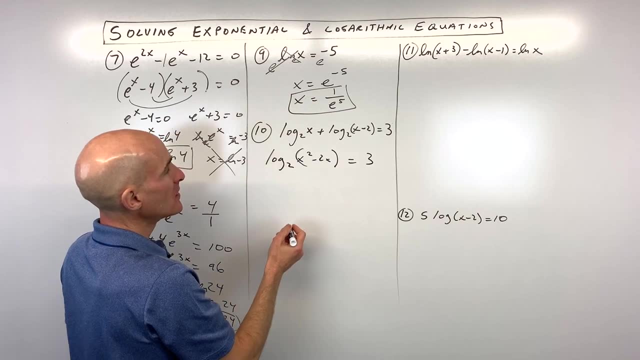 one log. So what we have is log base 2 of x times x minus 2, which comes out to x squared minus 2x equals 3.. So remember, when you add, you multiply. Now what we're going to do is we're going to. 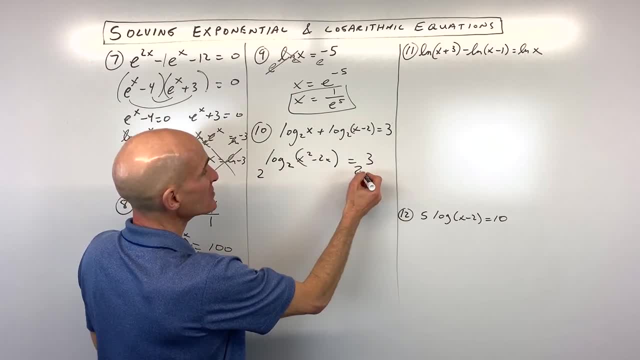 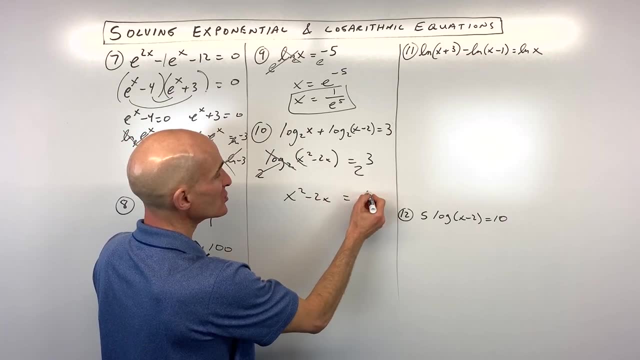 do the inverse of log base 2, which is to exponentiate both sides of the equation using base 2.. These are inverses. So that gives us x squared minus 2x equals 2x 2 cubed, which is 2 times 2 times 2,, which is 8.. Let's get everything on one side of the equation. 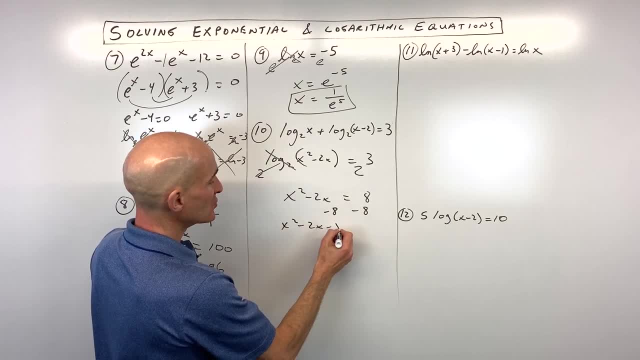 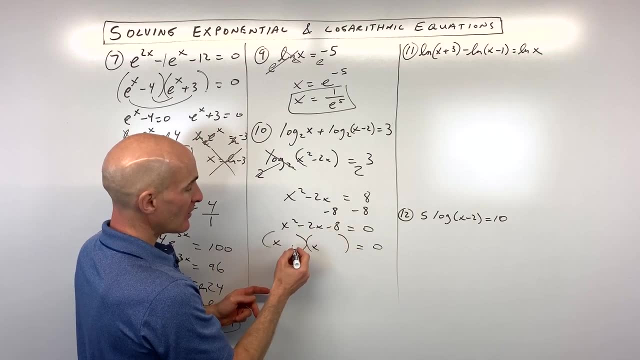 by subtracting 8 from both sides. So that's x squared minus 2x minus 8 equals 0. And now we're going to factor and set the factors to 0.. So what multiplies to negative 8 but adds to negative 2?? 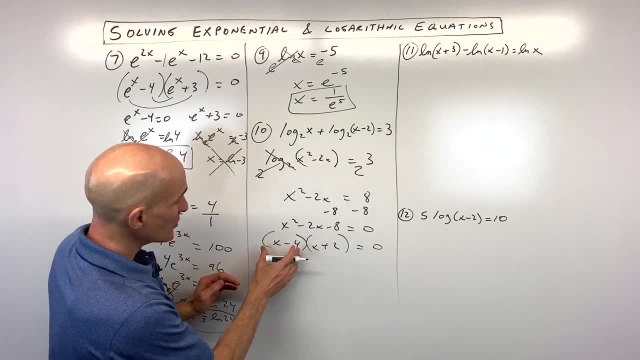 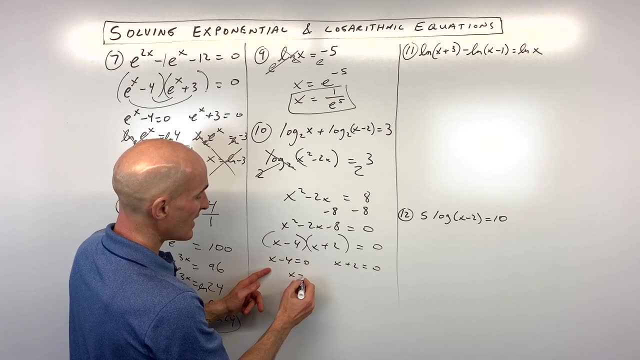 That's negative 4 and positive 2.. And then all we have to do is set each group equal to 0. So we have x minus 4 equals 0 and x plus 2 equals 0. Add 4 to both sides. 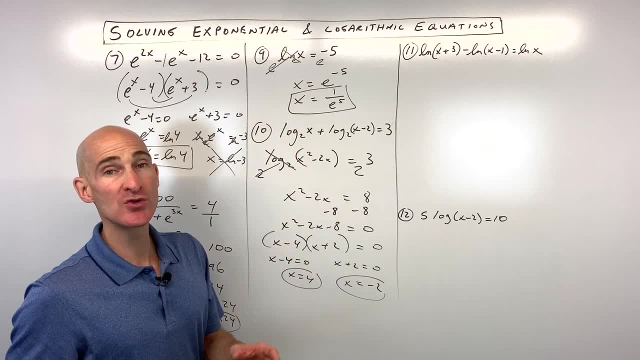 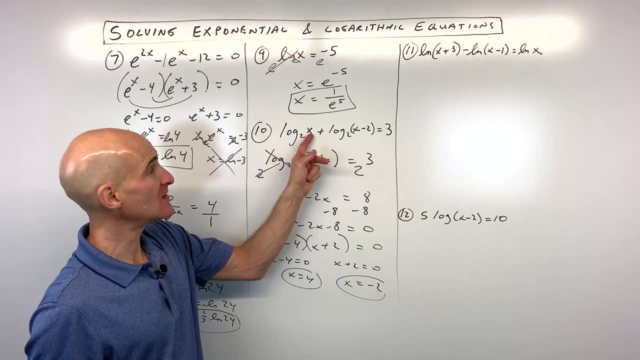 Subtract 2 from both sides. Now remember, when you solve these log equations you want to make sure that you're not getting any extraneous roots. So let's say, take this negative 2.. If we put negative 2 back in, we can't take the log of a negative quantity. That means that this is: 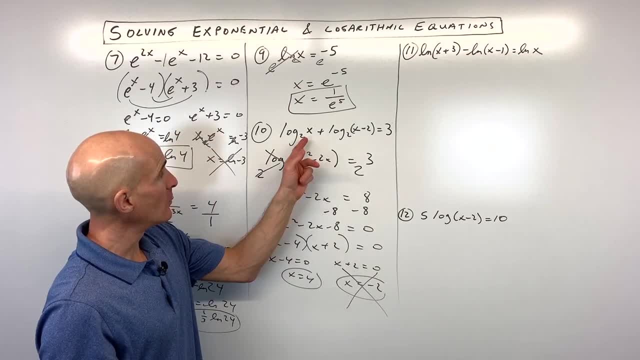 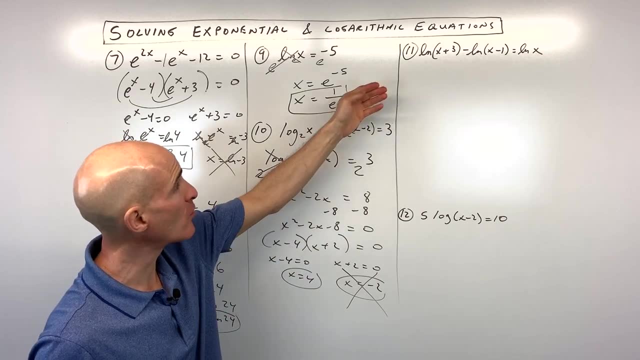 extraneous. Cross that one out. How about 4?? Well, this would be positive, This will be positive, So perfect. So it's just going to be x equals 4.. Okay, we've got a couple more examples here. 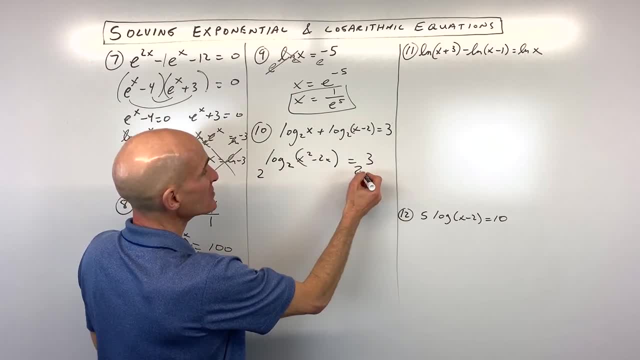 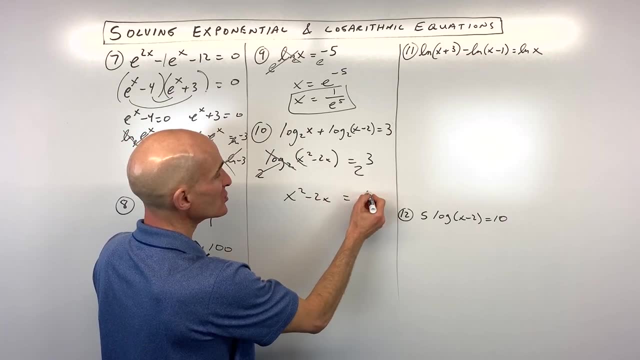 do the inverse of log base 2, which is to exponentiate both sides of the equation using base 2.. These are inverses. So that gives us x squared minus 2x equals 2x 2 cubed, which is 2 times 2 times 2,, which is 8.. Let's get everything on one side of the equation. 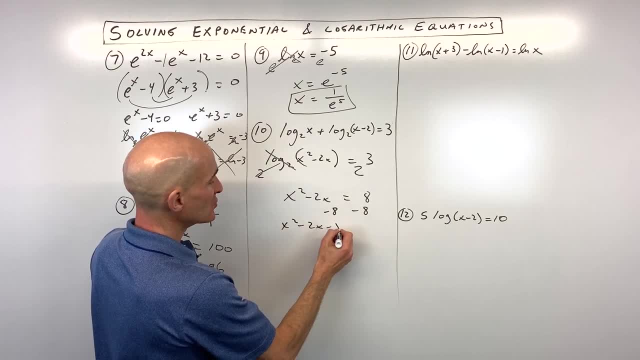 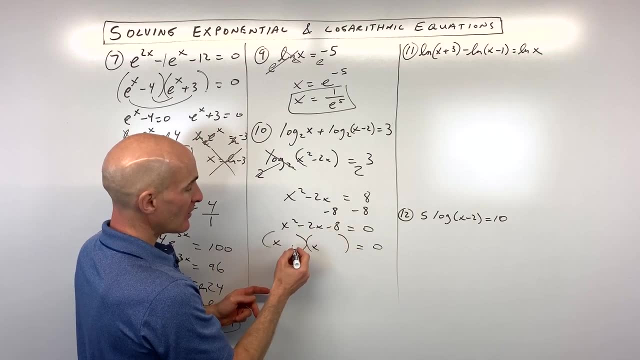 by subtracting 8 from both sides. So that's x squared minus 2x minus 8 equals 0. And now we're going to factor and set the factors to 0.. So what multiplies to negative 8 but adds to negative 2?? 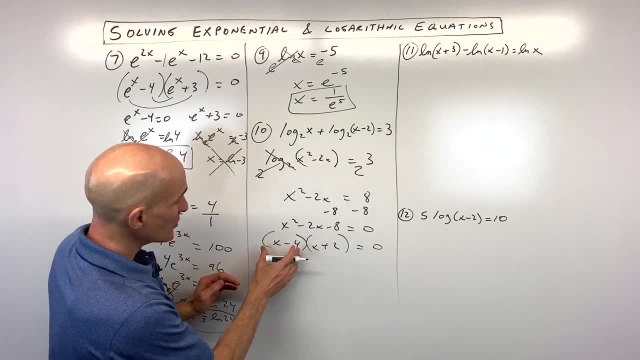 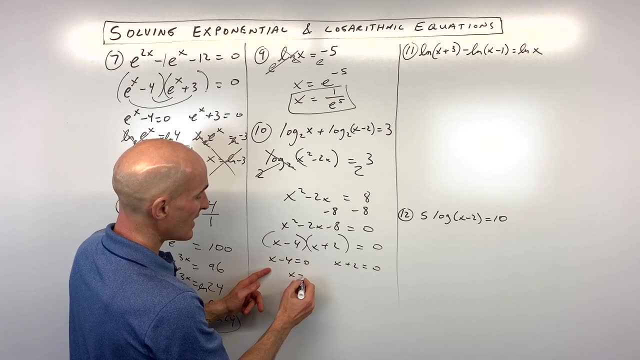 That's negative 4 and positive 2.. And then all we have to do is set each group equal to 0. So we have x minus 4 equals 0 and x plus 2 equals 0. Add 4 to both sides. 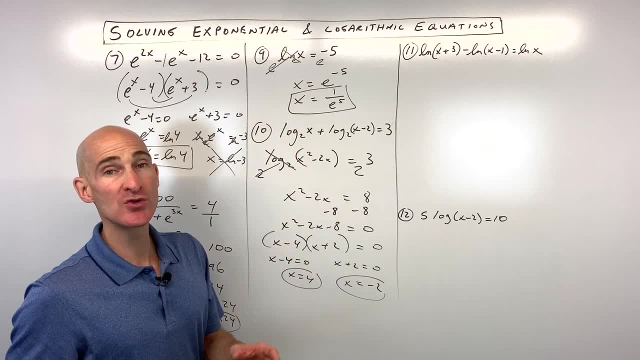 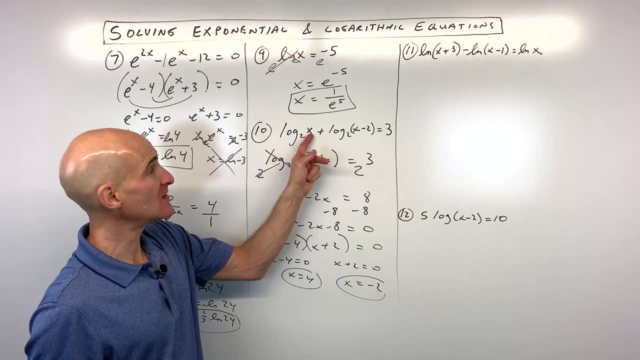 Subtract 2 from both sides. Now remember, when you solve these log equations you want to make sure that you're not getting any extraneous roots. So let's say, take this negative 2.. If we put negative 2 back in, we can't take the log of a negative quantity. That means that this is: 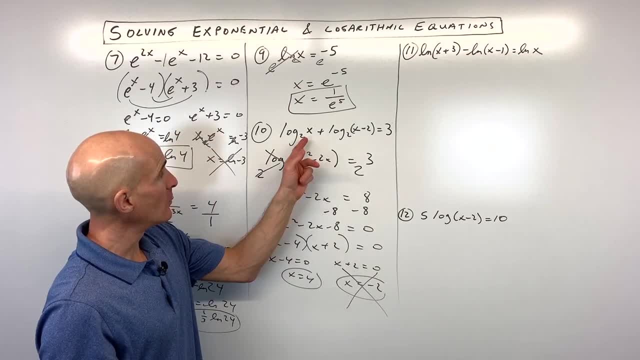 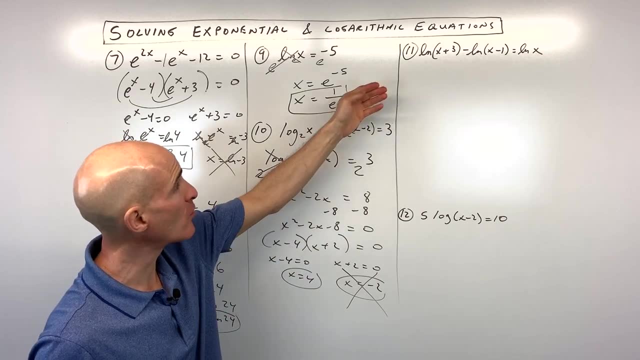 extraneous. Cross that one out. How about 4?? Well, this would be positive, This will be positive, So perfect. So it's just going to be x equals 4.. Okay, we've got a couple more examples here. 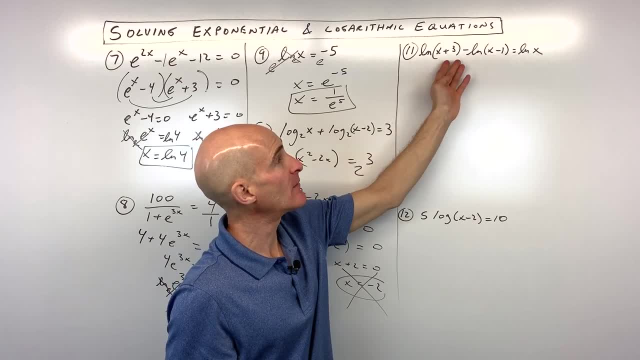 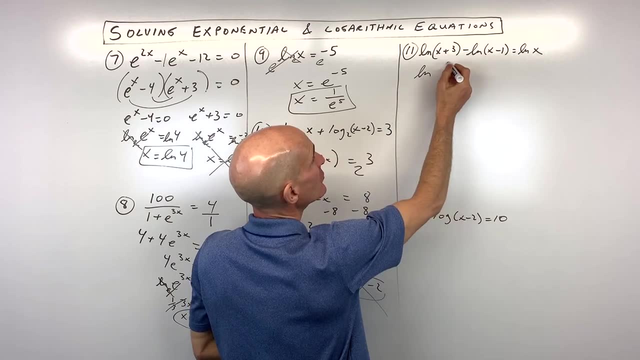 Number 11, a little bit more challenging Here. what I'm going to do is, again, I'm going to use properties for logs And remember, when you subtract, what do you do to the arguments? Remember you divide them right. So remember we're just combining these into one natural log. 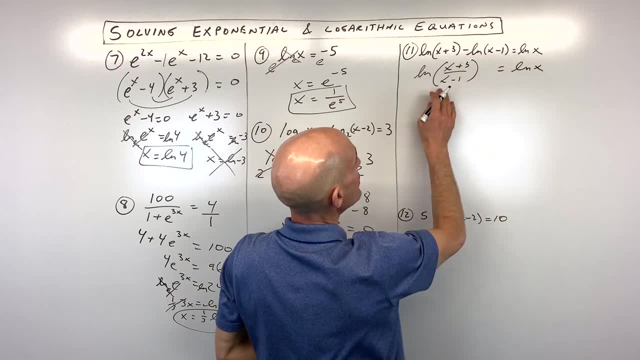 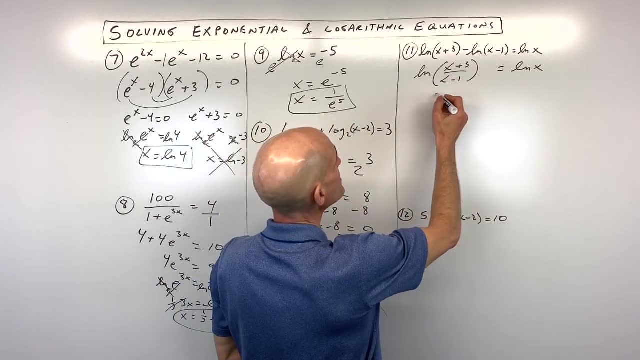 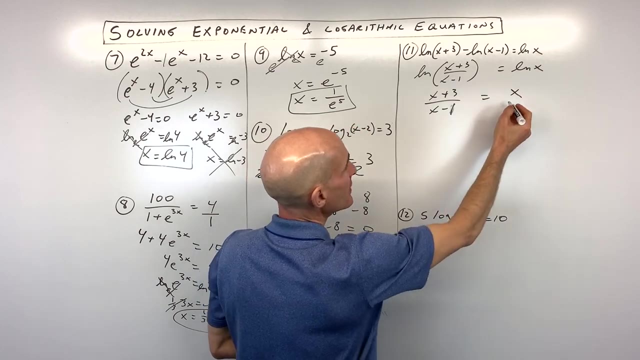 equals natural log of x. So here what we have: we have log base e, log base e. We can set the arguments equal to each other. This is called the one-to-one property of logs. So we're just left now with x plus 3 over x minus 1 equals x. You can think of x as x over 1.. You can think of x. 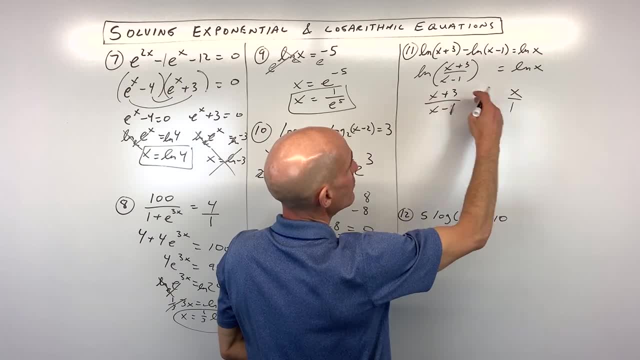 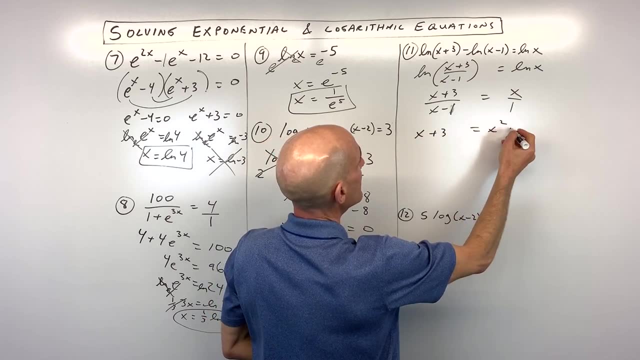 over 1, because anything divided by 1 is itself. And what we'll do is we'll cross multiply on the diagonal. using that means extremes, property and x squared minus x. So we're just multiplying Here. you want to make sure you distribute the x. Let's get everything on one side. So I'm going to 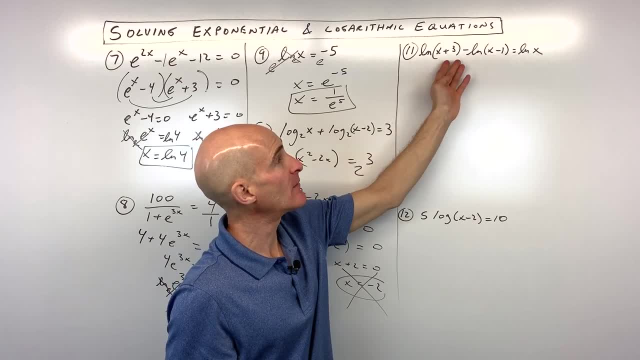 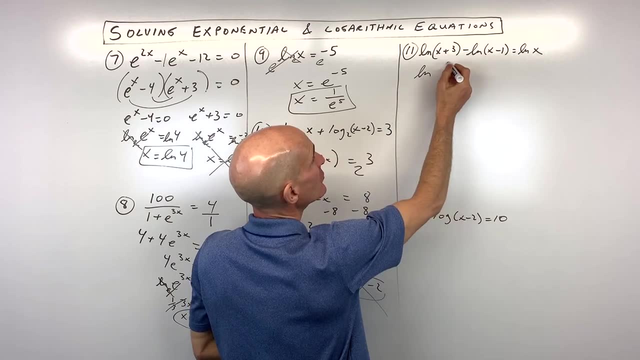 Number 11, a little bit more challenging Here. what I'm going to do is, again, I'm going to use properties for logs And remember, when you subtract, what do you do to the arguments? Remember you divide them right. So remember we're just combining these into one natural log. 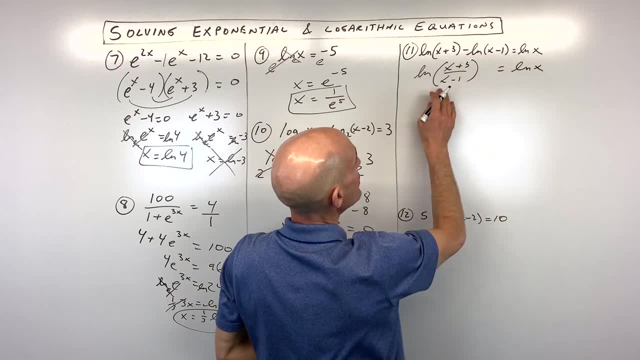 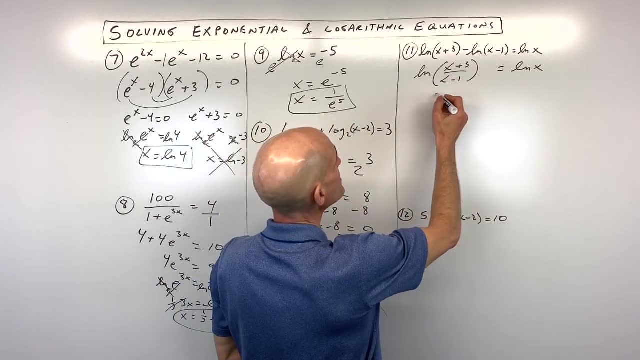 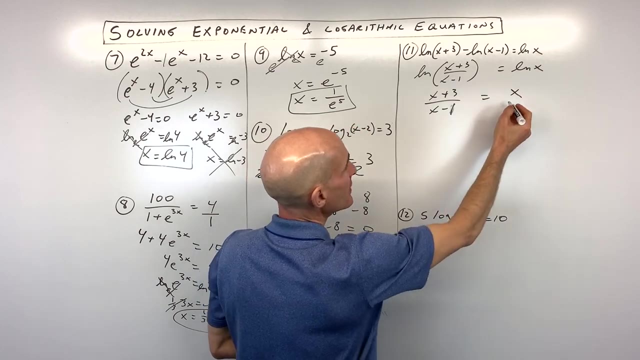 equals natural log of x. So here what we have: we have log base e, log base e. We can set the arguments equal to each other. This is called the one-to-one property of logs. So we're just left now with x plus 3 over x minus 1 equals x. You can think of x as x over 1.. You can think of x. 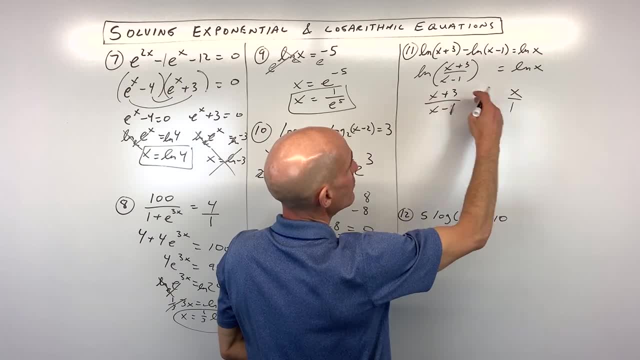 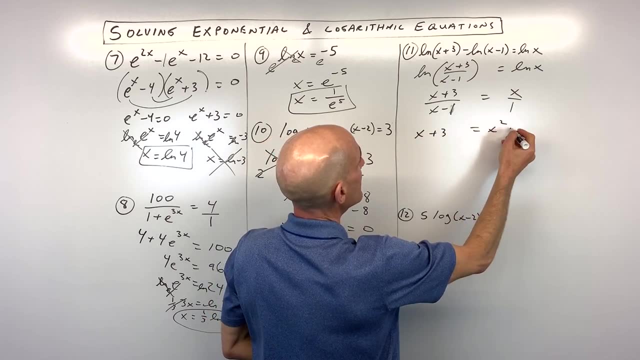 over 1, because anything divided by 1 is itself. And what we'll do is we'll cross multiply on the diagonal. using that means extremes, property and x squared minus x. So we're just multiplying Here. you want to make sure you distribute the x. Let's get everything on one side. So I'm going to 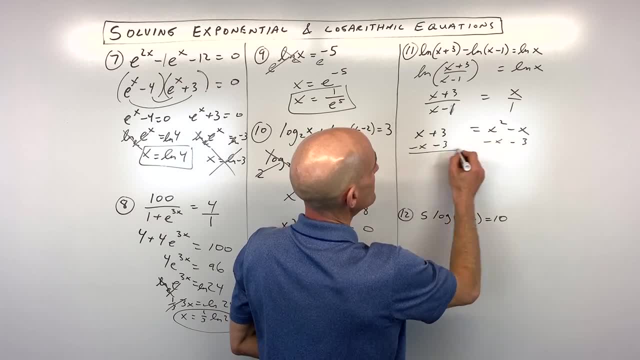 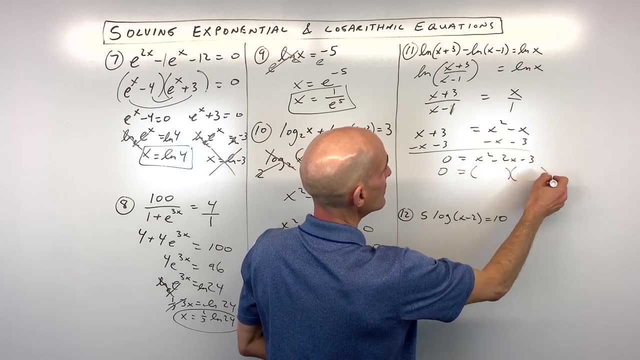 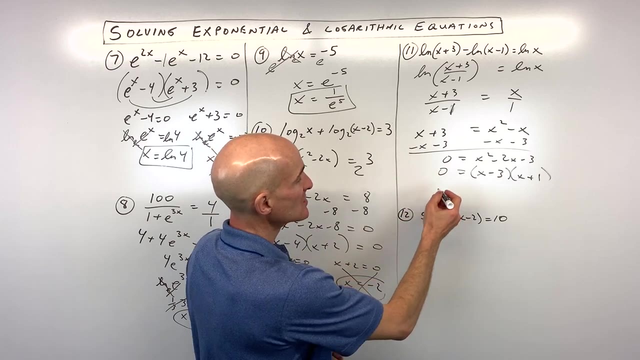 subtract x and subtract 3 from both sides. So that's going to give us 0 equals x squared minus 2x minus 3.. All we have to do now is factor and set the factors equal to 0. So this factors to x minus 3 and x plus 1.. If we set these factors to 0, we get 3 or negative 1.. 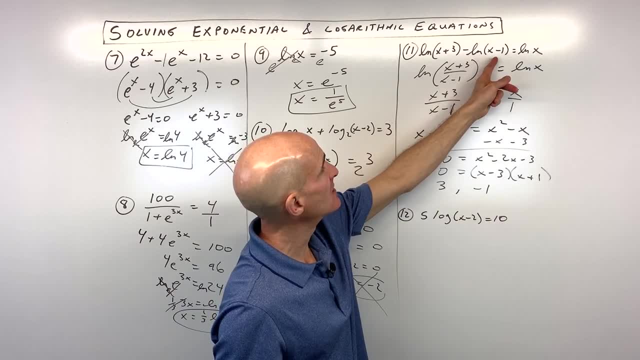 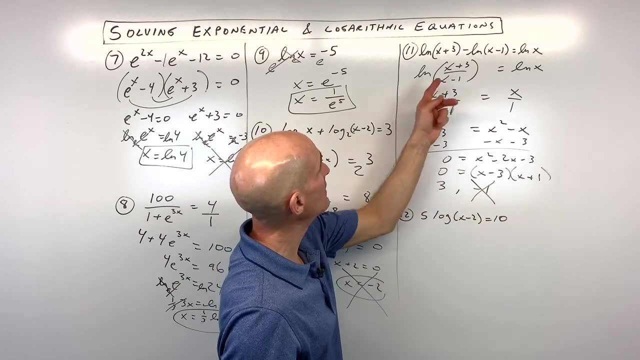 Now let's look at negative 1.. Negative 1 would make this negative. This would also make this negative. We can't take the log, or natural log of a negative quantity, So this is extraneous. Let's double check the 3.. This would be 6.. That's positive, That's good. 3 minus 1 is 2.. That's. 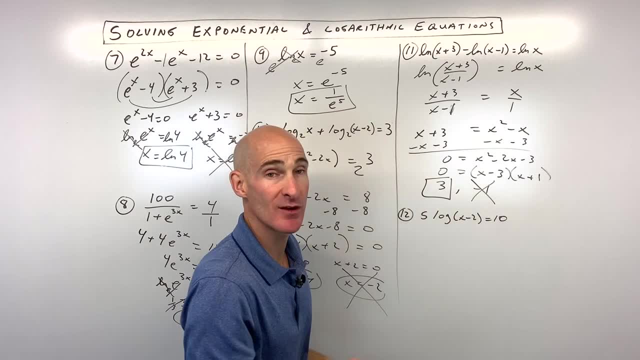 positive. That's good, And over there it's also positive, So it looks like it's just going to be 3.. OK, final question. See if you can do this one Here. we're trying to get, of course, x by its. 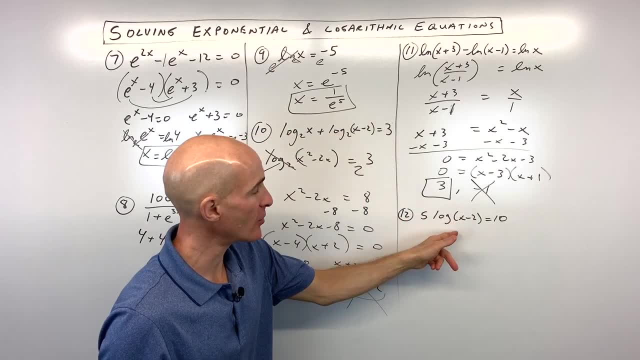 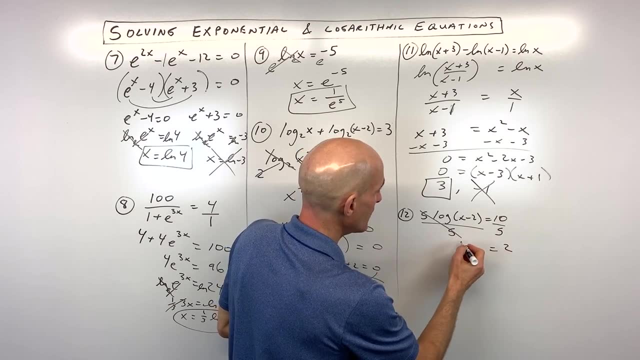 self thinking about working from the outside in towards that variable. What's the opposite of multiplying by 5?, Of course, dividing by 5, right, And so that's going to come out to 2.. And we have log And we don't see the base. So when the base isn't written, it's understood to be base 10.. So 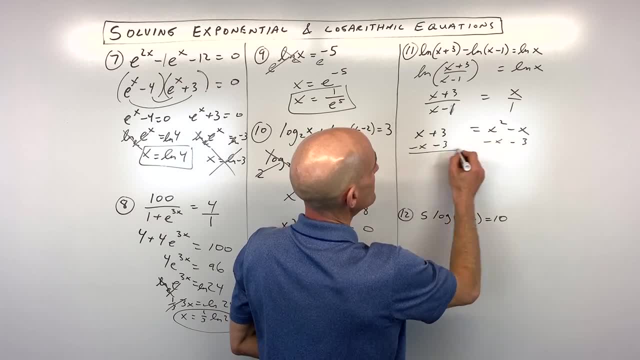 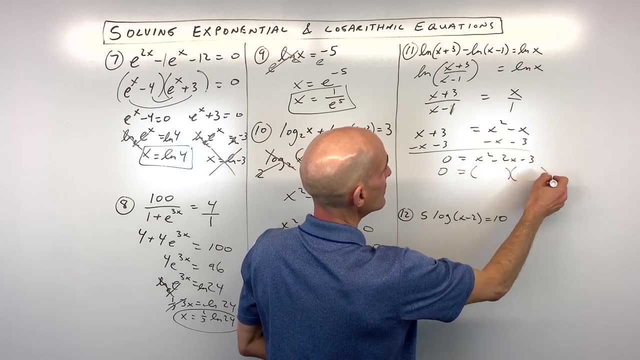 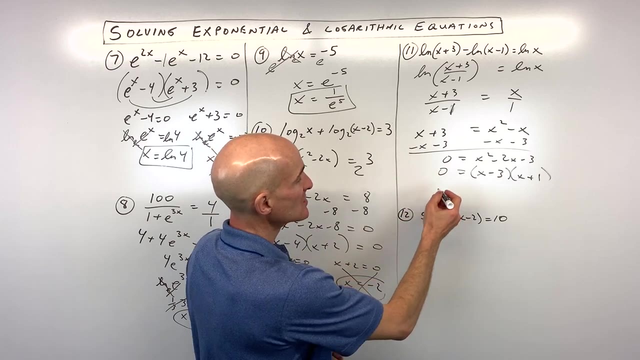 subtract x and subtract 3 from both sides. So that's going to give us 0 equals x squared minus 2x minus 3.. All we have to do now is factor and set the factors equal to 0. So this factors to x minus 3 and x plus 1.. If we set these factors to 0, we get 3 or negative 1.. 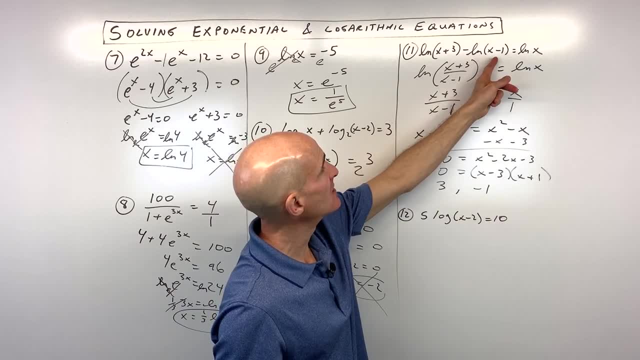 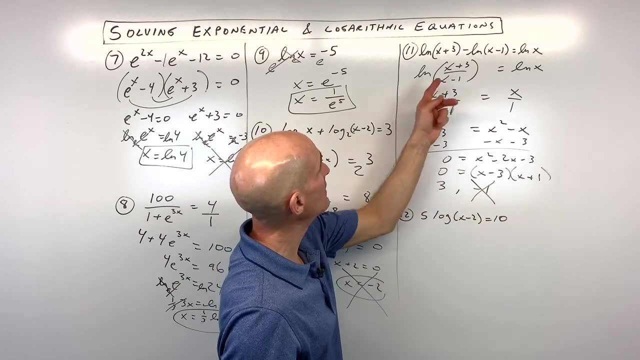 Now let's look at negative 1.. Negative 1 would make this negative. This would also make this negative. We can't take the log, or natural log of a negative quantity, So this is extraneous. Let's double check the 3.. This would be 6.. That's positive, That's good. 3 minus 1 is 2.. That's. 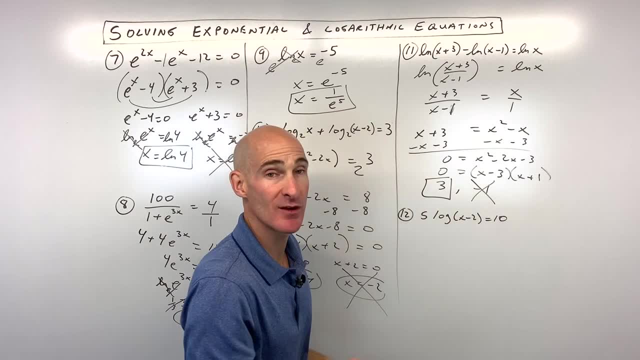 positive. That's good, And over there it's also positive, So it looks like it's just going to be 3.. OK, final question. See if you can do this one Here. we're trying to get, of course, x by its. 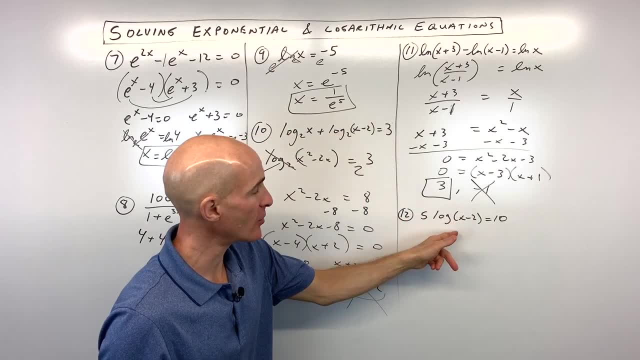 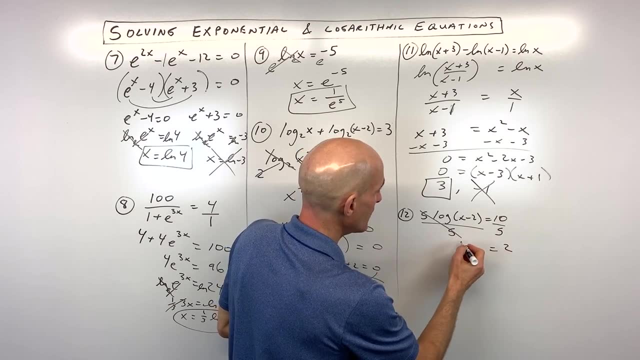 self thinking about working from the outside in towards that variable. What's the opposite of multiplying by 5?, Of course, dividing by 5, right, And so that's going to come out to 2.. And we have log And we don't see the base. So when the base isn't written, it's understood to be base 10.. So 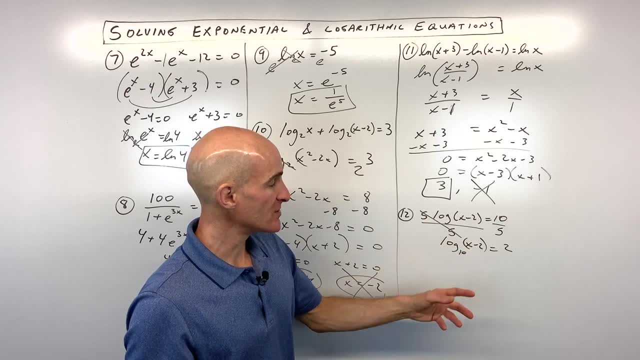 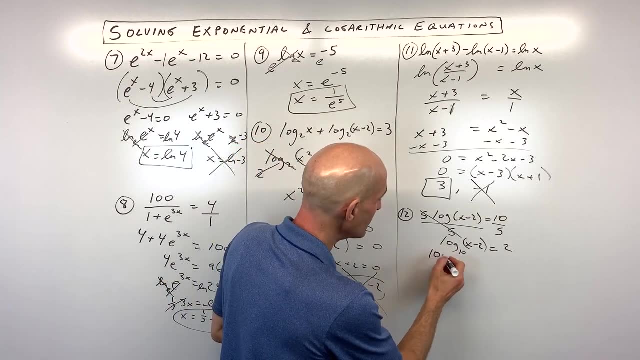 I'll just pencil that in for us. And now, because that variable is like inside of that log, we want to get it by itself or isolate it by doing the inverse. So instead of log base 10, let's exponentiate both sides using base 10.. Those are inverses. 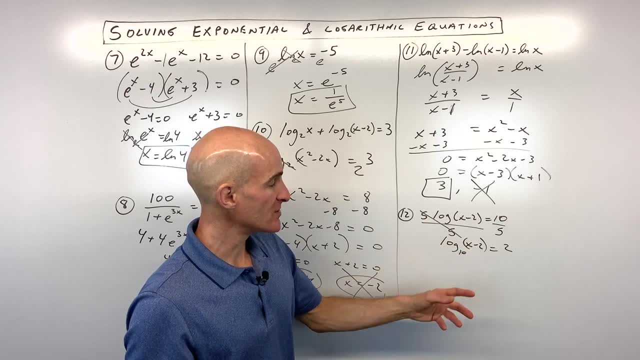 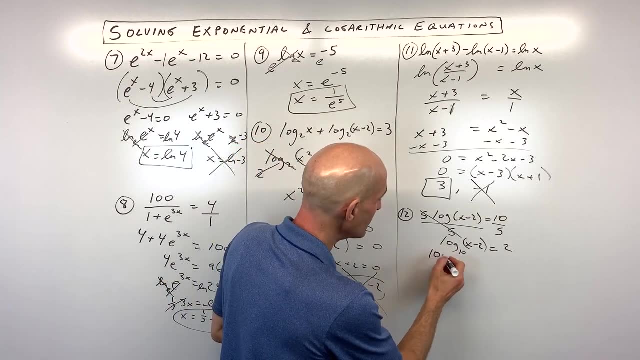 I'll just pencil that in for us. And now, because that variable is like inside of that log, we want to get it by itself or isolate it by doing the inverse. So instead of log base 10, let's exponentiate both sides using base 10.. Those are inverses. 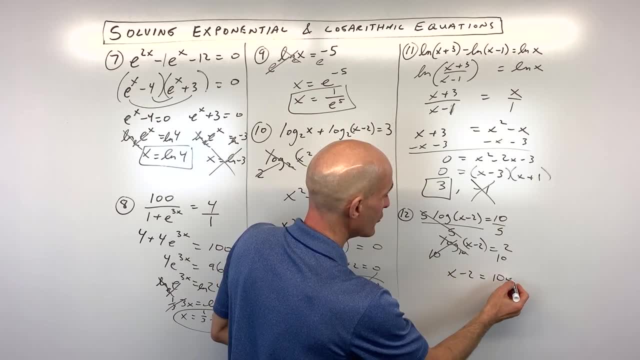 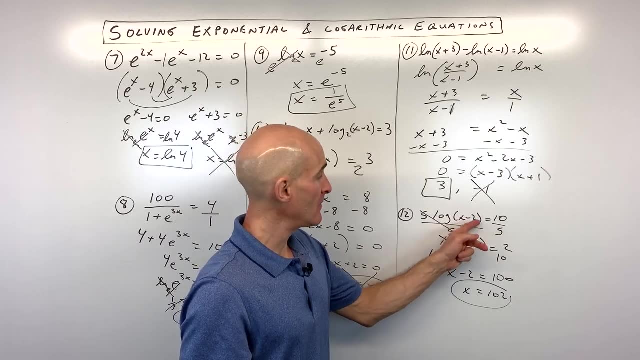 We have: x minus 2 equals 10 squared, which is 10 times 10, or 100.. Add 2 to both sides And you can see x comes out to 102.. Quickly go ahead and put it back in. Make sure you're taking the log of a. 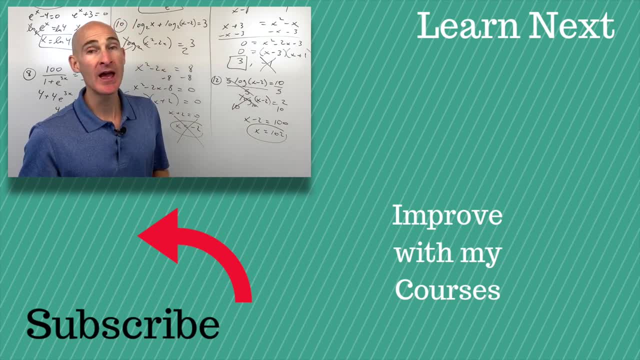 positive quantity, And that is So. that's our final result. If you want to learn more about logarithms, follow me over to that video right there where I go into rewriting logs in exponential form: solving logarithmic equations, graphing logs. Follow me over there, We'll dig into some. logs: Thank you,